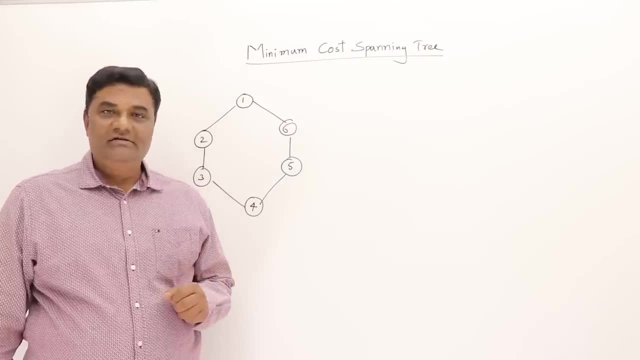 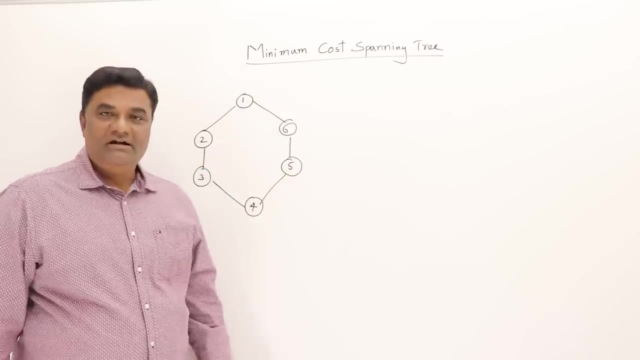 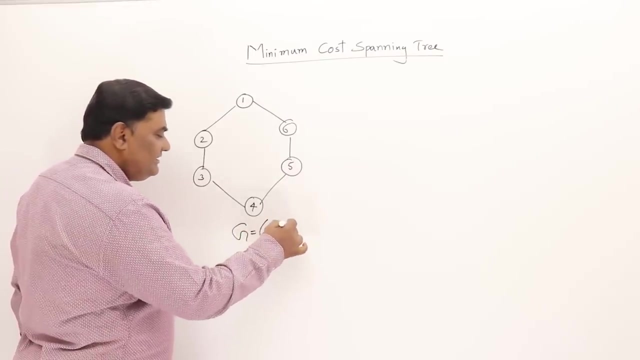 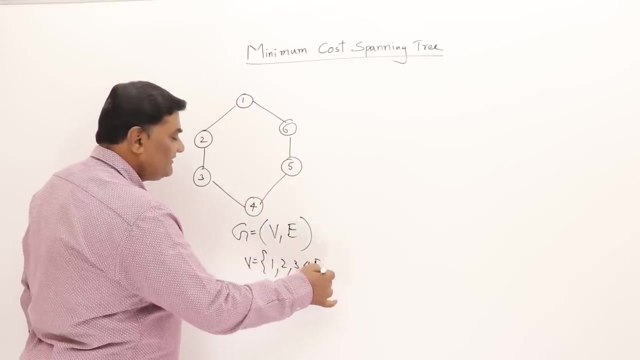 The topic is minimum cause: spanning tree. So for that, first of all, we will understand what does it mean by a spanning tree? Here I have an example graph. Graph is represented as G and VE. V is the set of vertices, 1,, 2,, 3,, 4,, 5,, 6 and E is the set of edges. The set of edges are from 1 to. 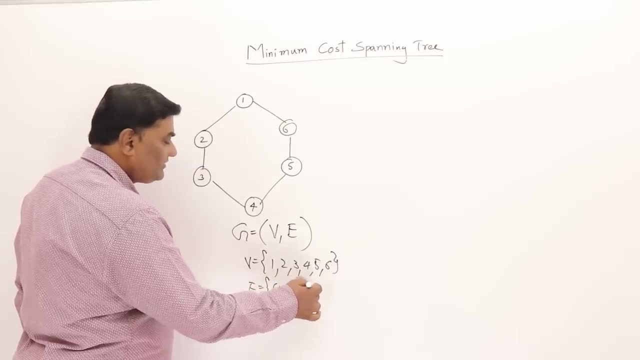 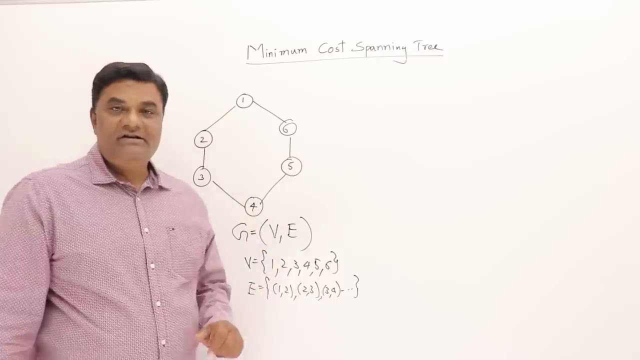 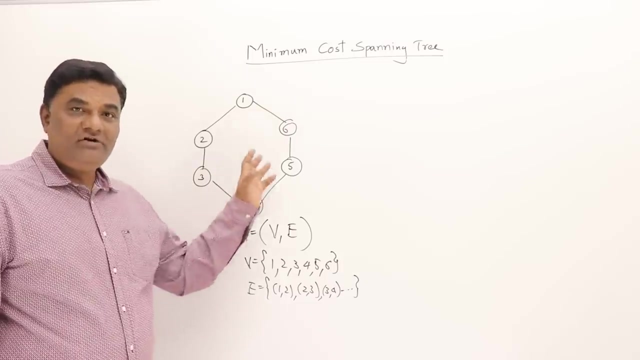 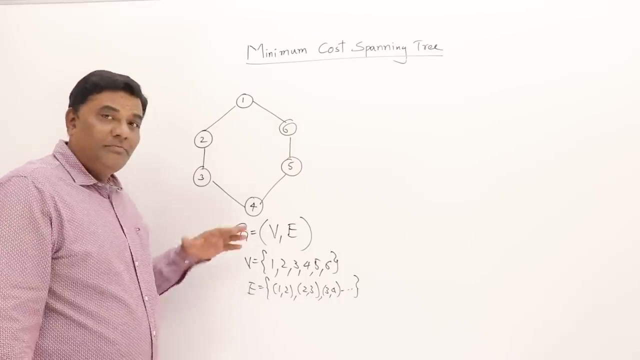 2 and 2 to 3, 3 to 4 and so on. Graphs are represented as set of vertices and edges. Now, what is this? spanning tree? Spanning tree is a subgraph of a graph. I should take the subset of this. So, subset of what? Vertices and edges? Both the subset or only one subset? So I should take the subset of edges. 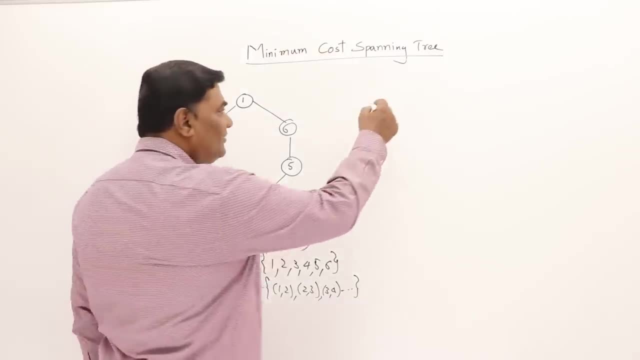 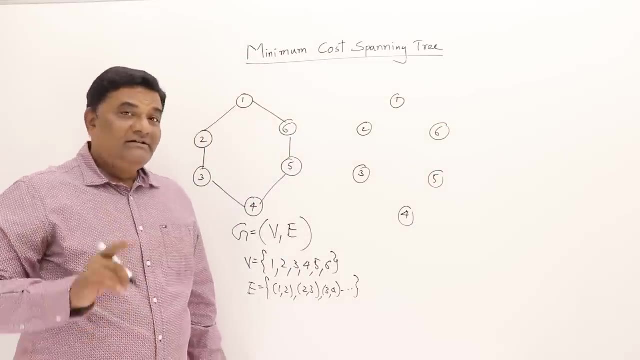 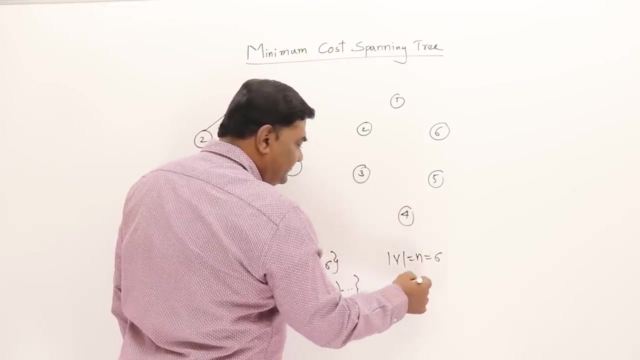 Vertices must be as it is, So I should take all vertices 6.. Spanning tree means I should take all vertices. Then how many edges, How many vertices I have? Number of vertices are n, that is 6.. So I should take number of vertices minus 1, that is only 5 edges. 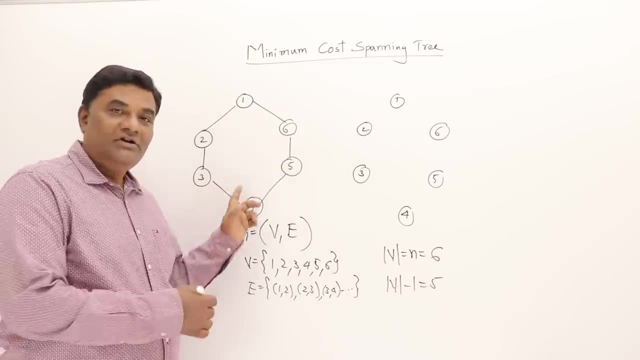 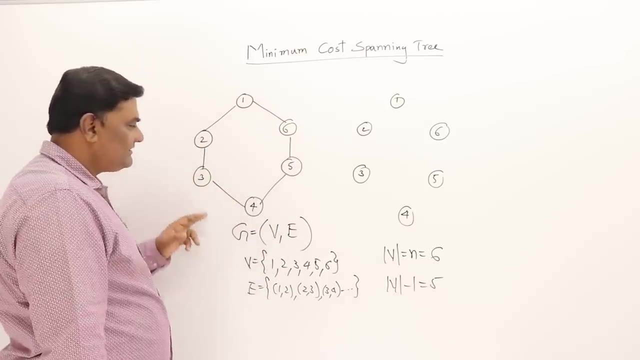 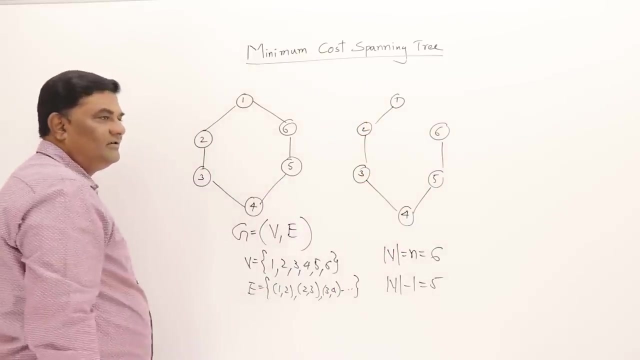 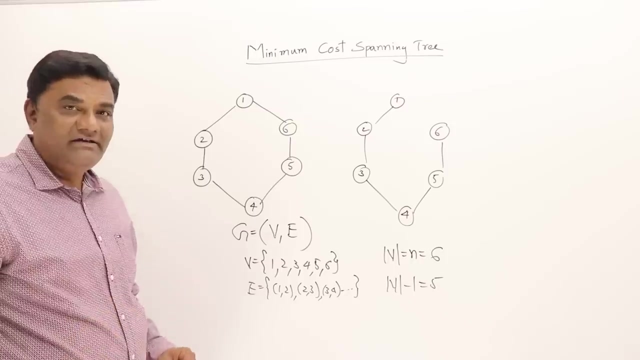 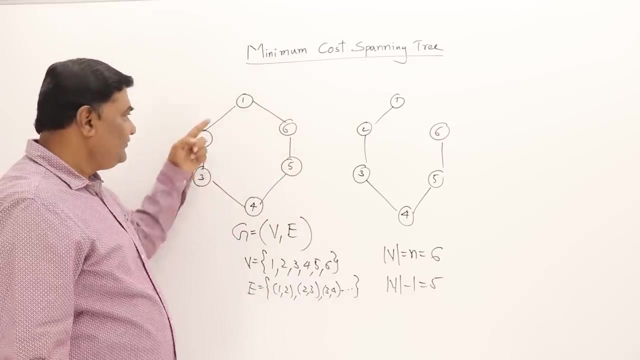 Spanning tree is a subgraph of a graph having all vertices but only n minus 1 edges. So out of these edges I should take only 5.. So 1,, 2,, 3,, 4, 5.. I did not take this one. So this is a spanning tree. See, a tree will not have a cycle, So there is no cycle here. Yes, there is no cycle here. If I this, you can say it is a cycle. If you start from one vertex you can again reach back to that vertex. But here 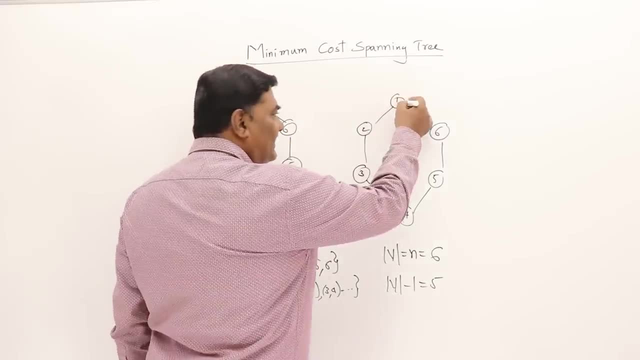 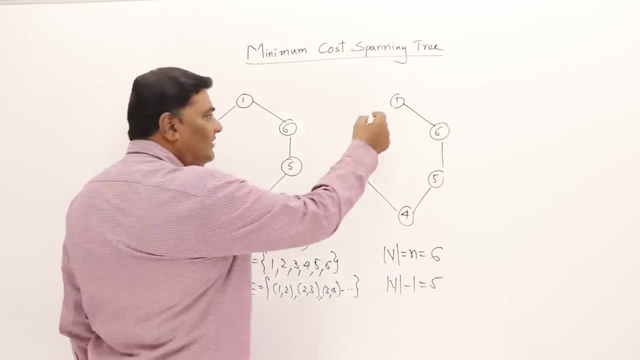 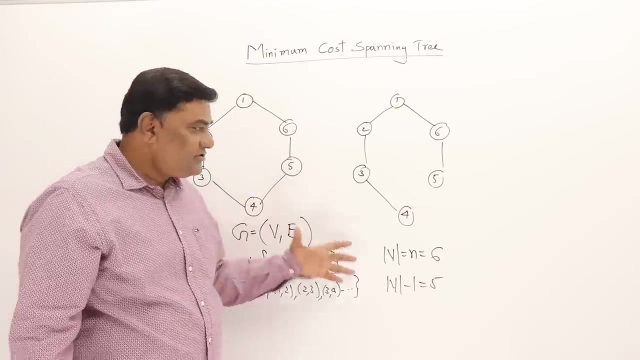 there is no cycle. is it possible that I will take this one, but I will not take this? yes, there's also a spanning tree. I will take this, but I will not take this. yes, this is also a spanning tree. so which edge to select? that is a choice. 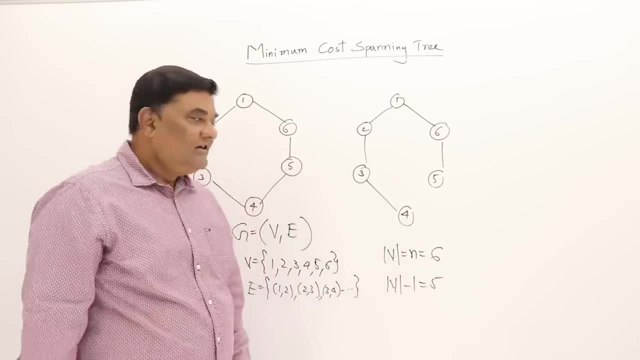 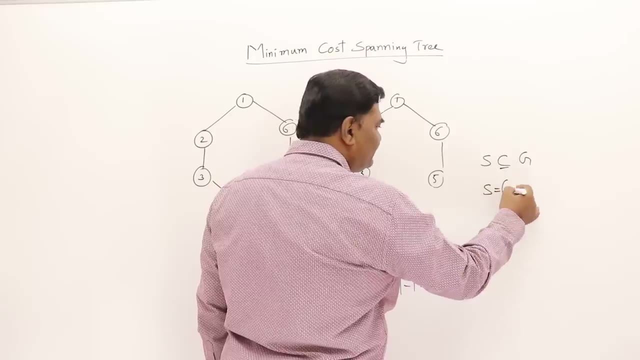 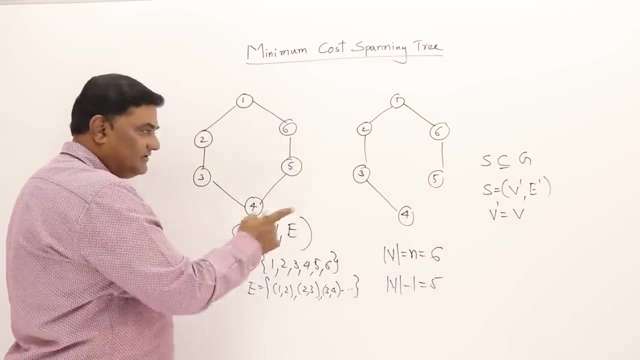 that's a choice for a spanning tree. so I can say that S is a subgraph of a graph where S is defined as set of vertices and set of edges, where set of vertices are same as the vertices of a graph and edges are number of vertices minus 1. so 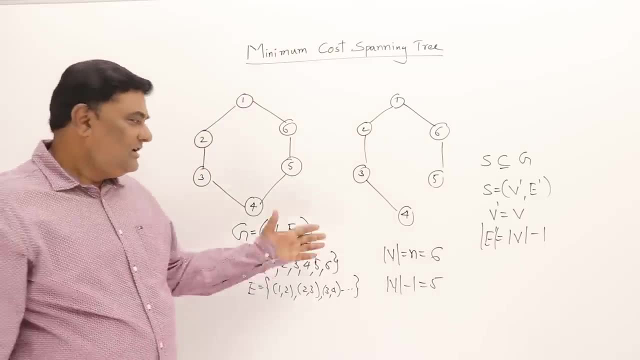 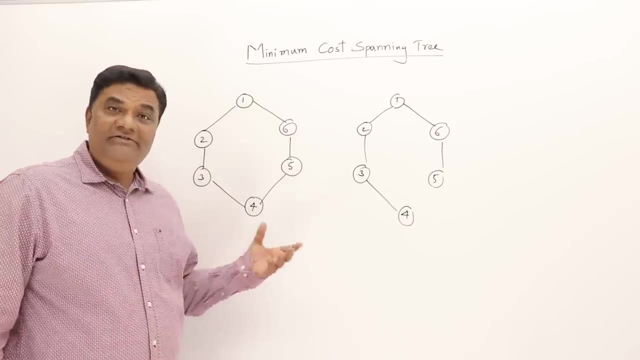 the number of edges are number of vertices minus one. this how formally we can divide, and mathematics we can define like this: our next thing: for a given graph, how many different spanning trees can be generated? I won't give you an answer. answer. I won't give you an answer. answer. 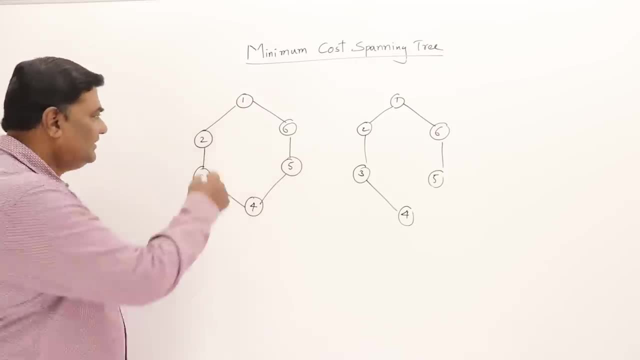 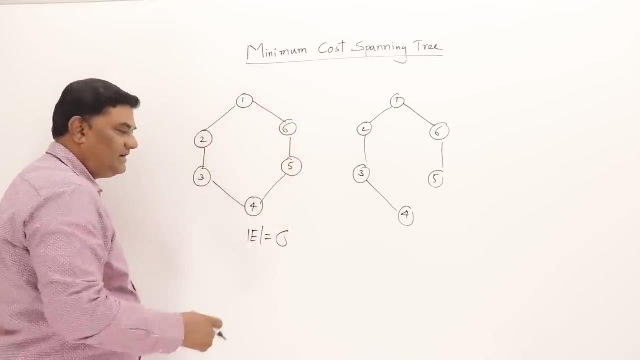 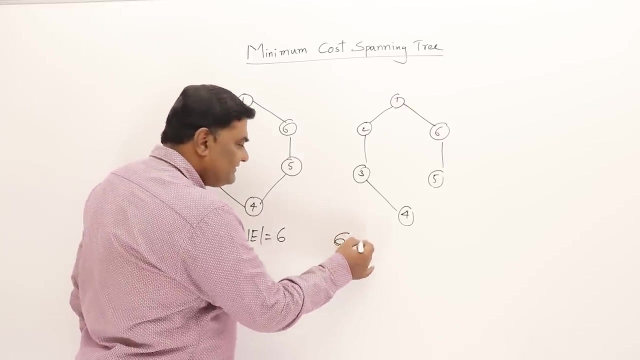 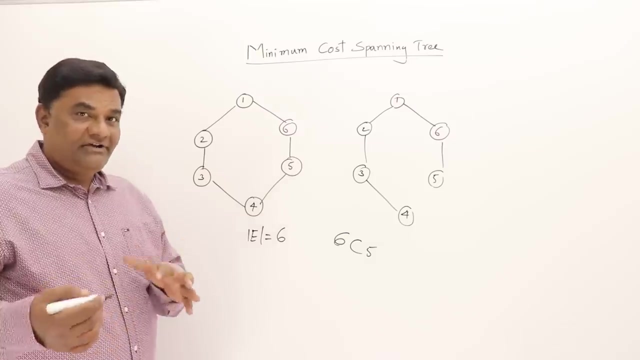 I won't give you an answer. answer to know that how many different spanning trees are possible. so see, number of edges are how many? six, one, two, three, four, five, six i have in a spanning tree? i should take only five. i should take only five. so six c, five out of six edges. out of six edges, i have to select five. 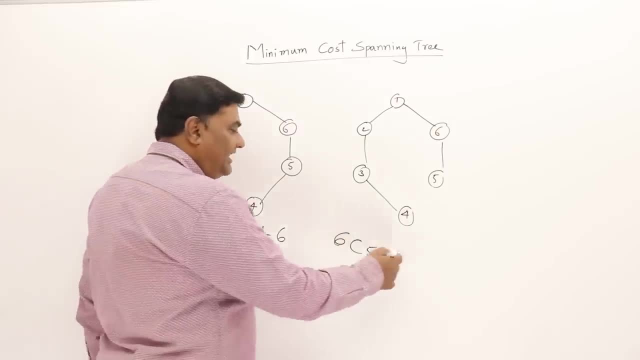 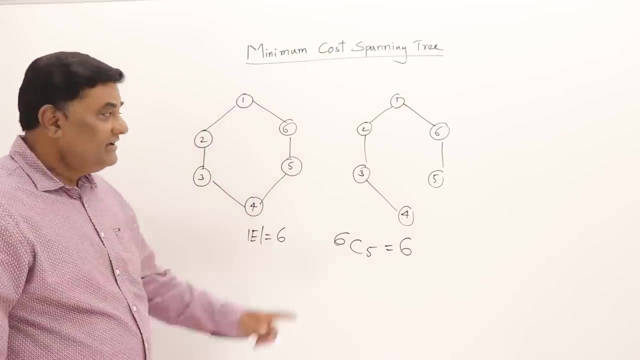 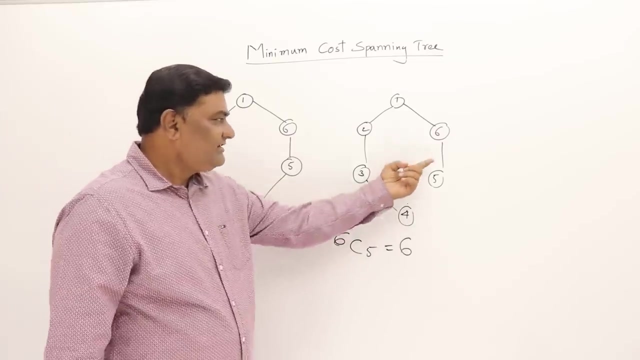 how many ways i can do that. so six, five c ways. so fix six five c is how much six only so i can have six different spanning trees. just now, you can see, it is a simple one that i have skipped this edge. like this, i can leave one, one edge right and again form a spanning tree right. i can take all except. 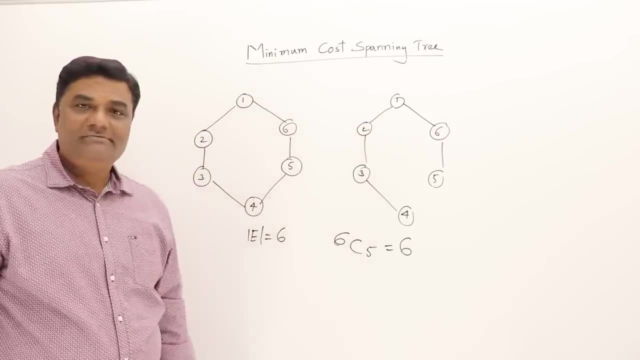 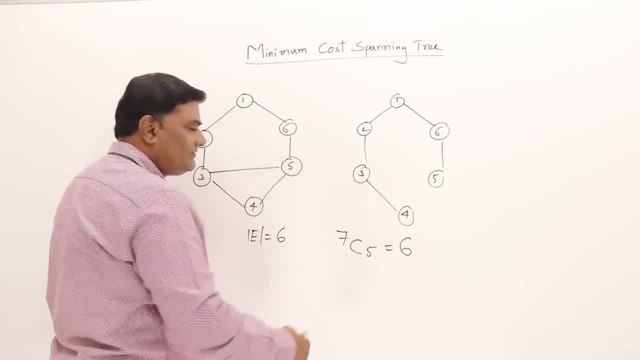 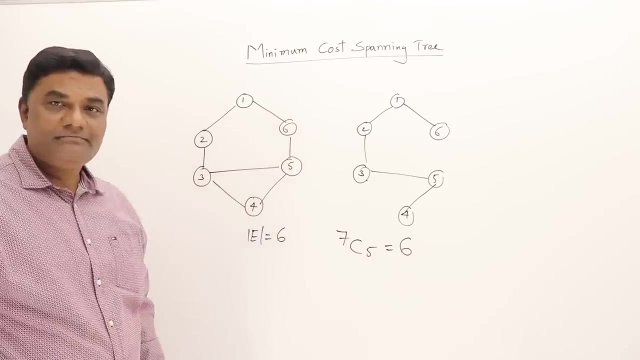 this: take all except this. take all except six are possible, suppose, if i have one more edge now. idor dragon have two edges now. now i have seven edges and i want to select five. now how many spanning trees are possible? see, i have this spanning tree also, or i can have this spanning. 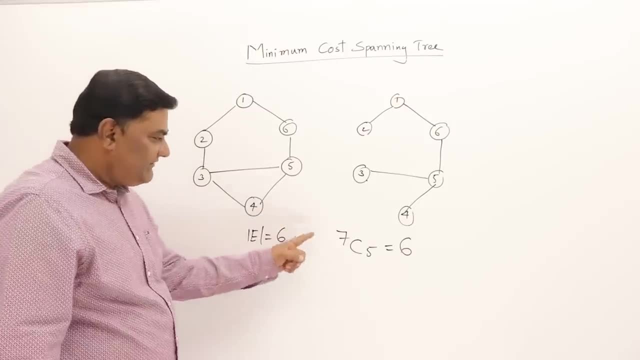 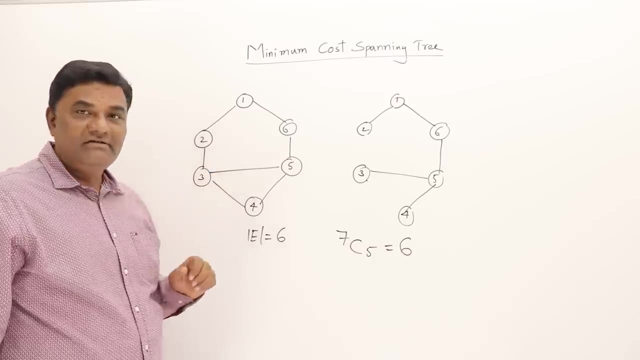 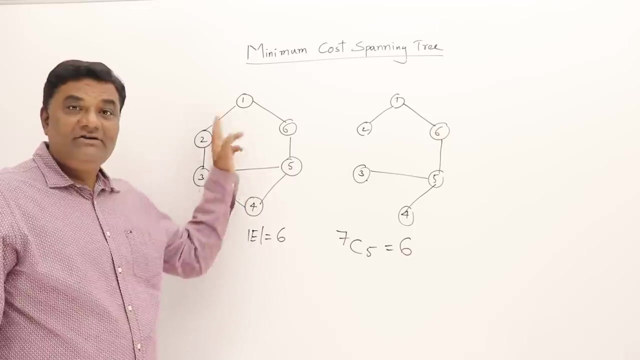 tree also. now possibilities are more. now this is 7c5, 7c5, but this edge will form cycle. so how many cycles it is forming? this is one cycle and this is c5 and is another cycle. so this edge is forming two cycles of number of vertices: less than six. 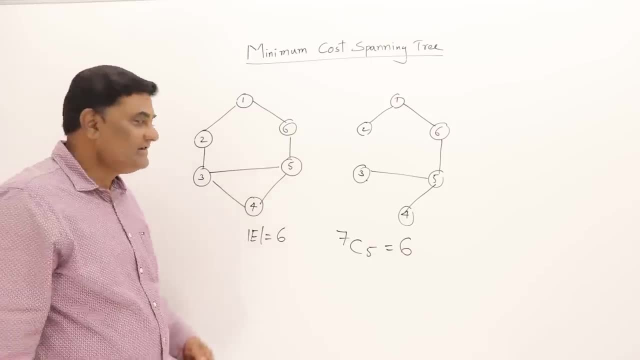 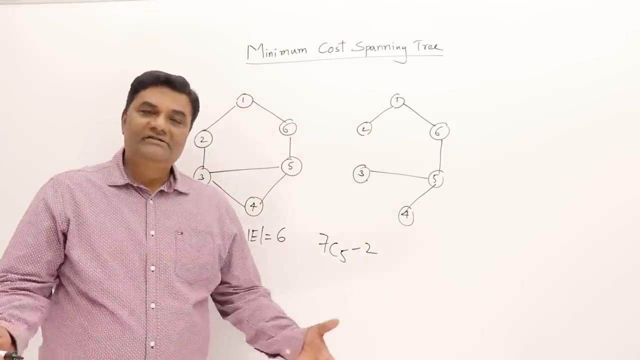 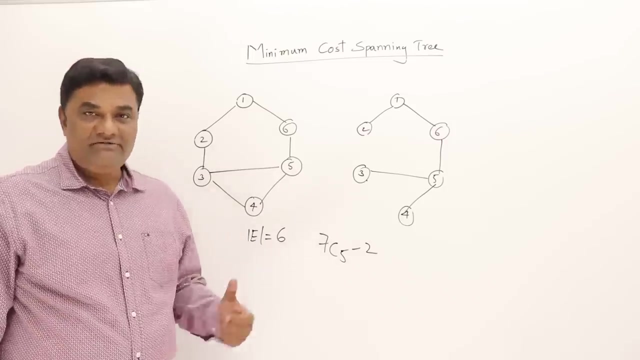 so if it is forming number of vertices less than six, then you will be 7c5 minus 2. so that's it. so what's the formula to know how many different spanning trees are possible from a given graph? so, whatever the number of edges you have, you should take all those. 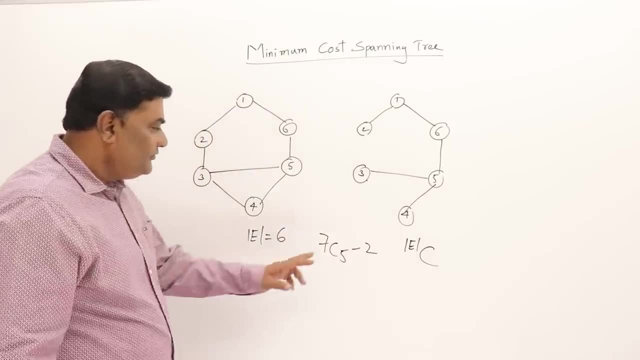 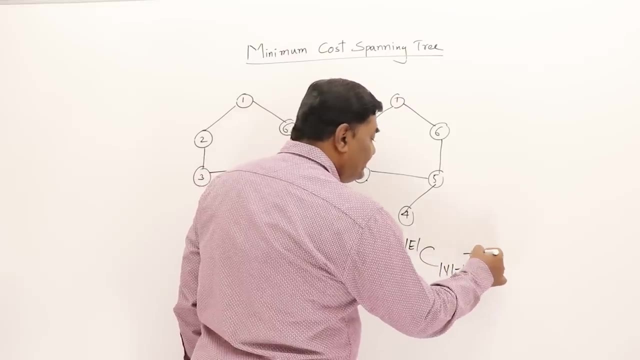 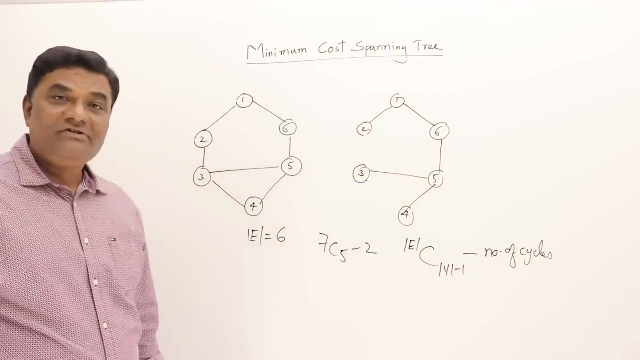 and see of how many edges you need. you need 5. so 5 is what? number of vertices minus 1? so this is number of vertices minus 1 and minus number of cycles. you have to subtract number of cycles. i have a graph where the edges are having weights. 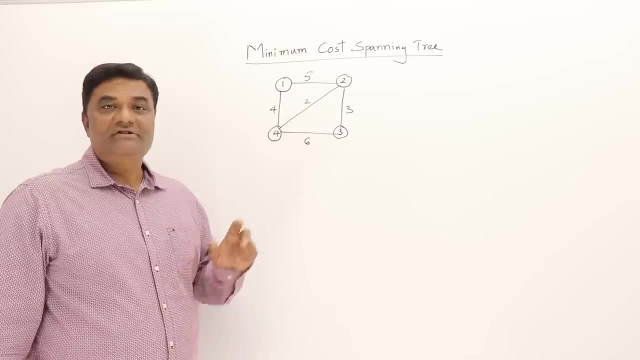 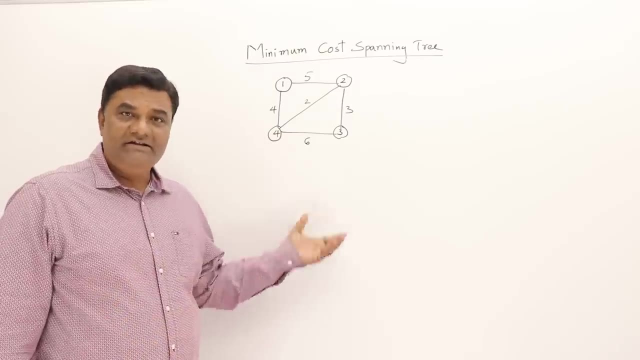 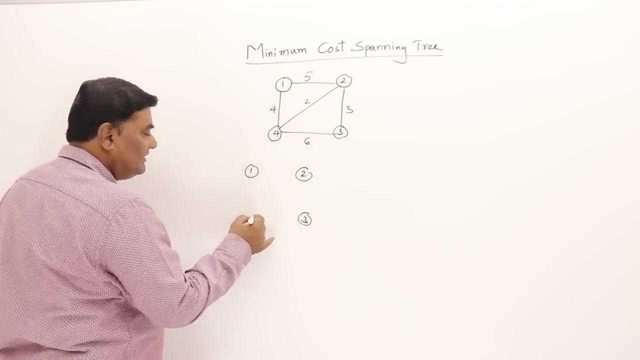 so this is a weighted graph. this is a weighted graph. i want to know what are the spanning trees possible, so I'll draw few spanning trees. let us draw one spanning tree. this is vertex 1 and 2 and 3 and 4. so 4 vertices are there then. how many? 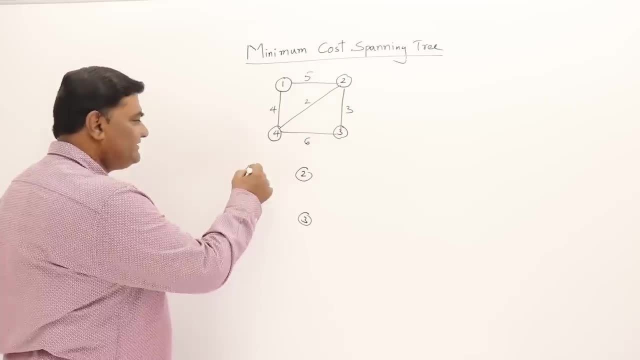 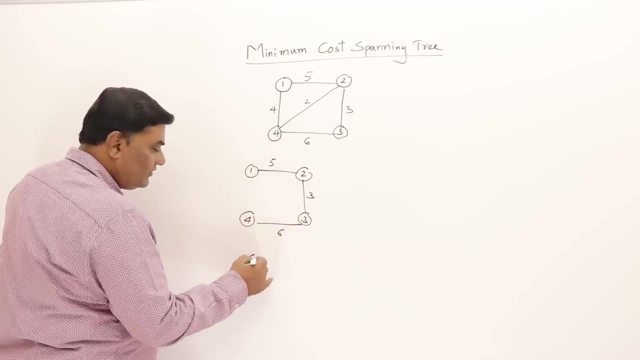 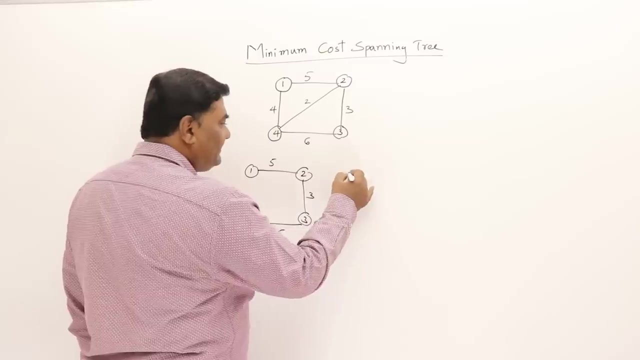 edges. I should take 4 minus 1, only 3. so I'll select this one: 1, 2, 3. so what is the weight of this one? 5, 3 and 6. so what is the cost of this spanning tree? cost of this spanning tree is 14. I'll take one more spanning tree- 1, 2, 3, 4- and I'll 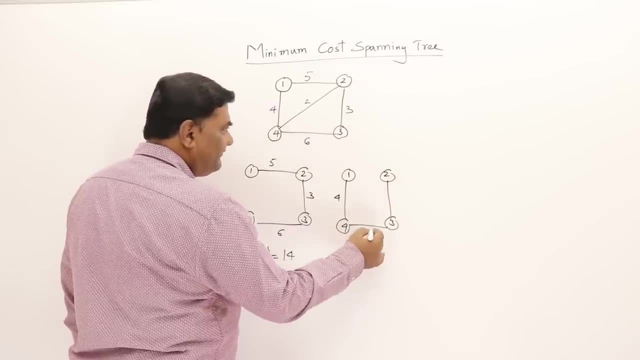 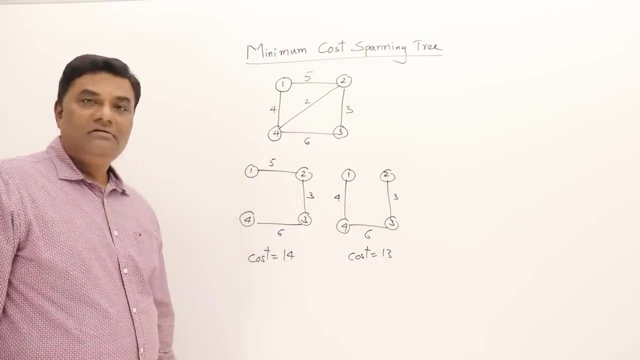 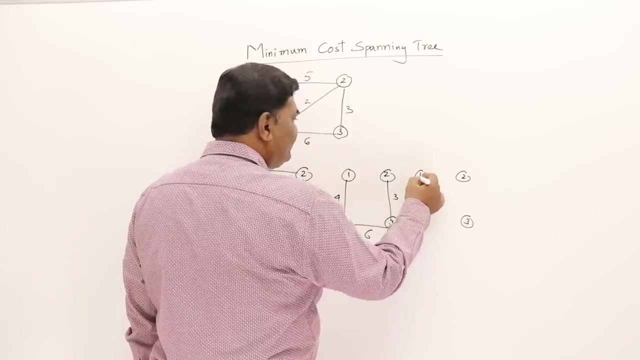 take these edges. let us see what is the cost of this: 4, 6, 3. then what is the cost of this one, 13? I'll take one more spanning tree: 1, 2, 3, 4, and I'll take these edges, this one and this one and this one. 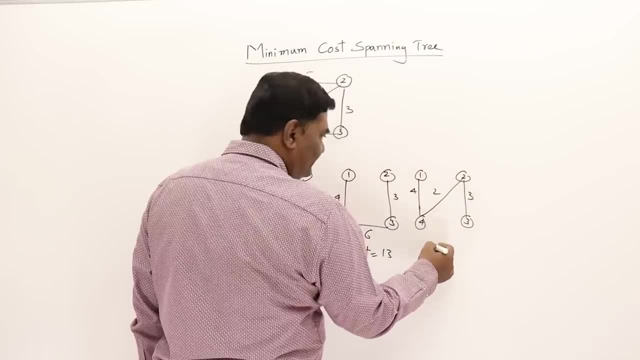 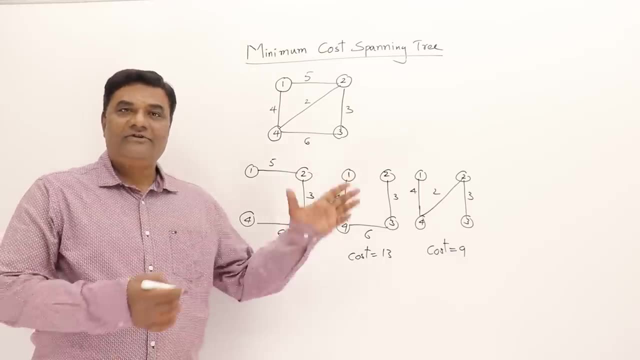 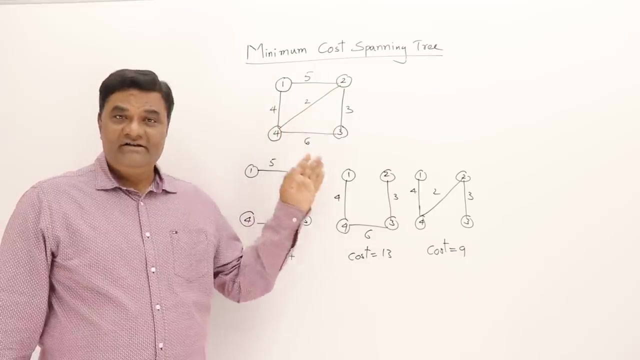 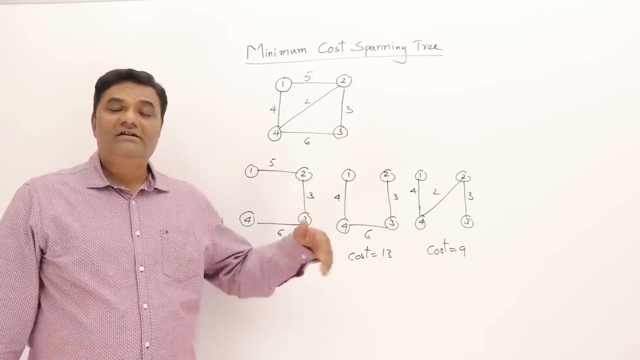 4, 2 and 3. so this is cost. is how much nine? now from this example, some observation. we can understand something. if you have a weighted graph and you get different spanning trees, the cost of the spanning trees may be varying. you can get a different cost of spanning trees. now the 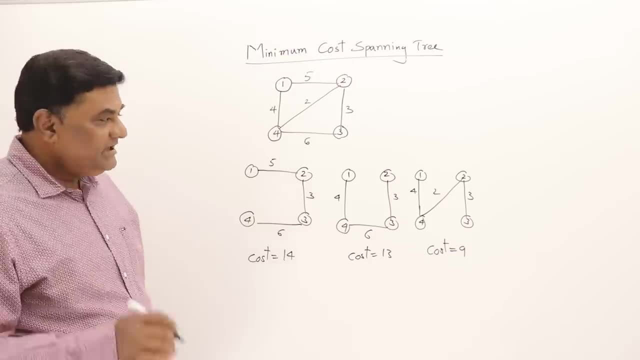 problem is that we have a spanning tree and the cost of the spanning trees may be varying. you can get a different cost of spanning trees. now the problem is that is, can I find out the minimum cost spanning tree? can I find out the minimum one which gives me? 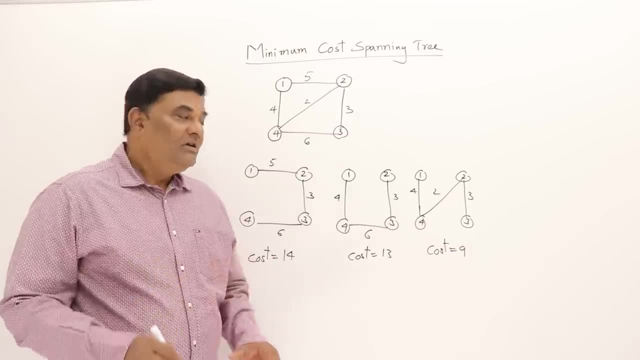 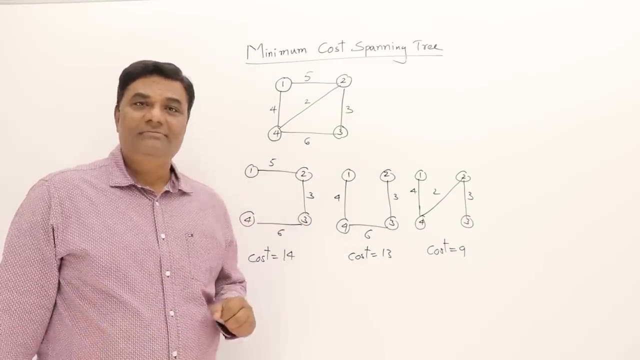 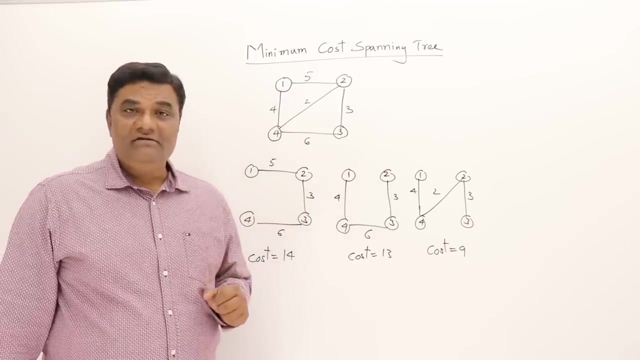 minimum? yes, you can find out how you can try all possible spanning trees and then from that you can check whichever is minimum. you can pick up that answer. this is one method. trying all possible spanning trees will be too lengthy. is there any greedy method? yes, the greedy methods are available. 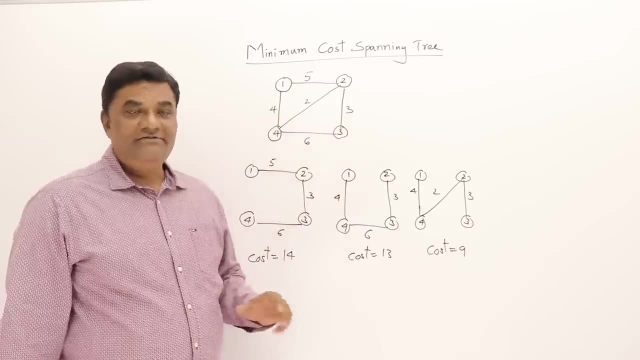 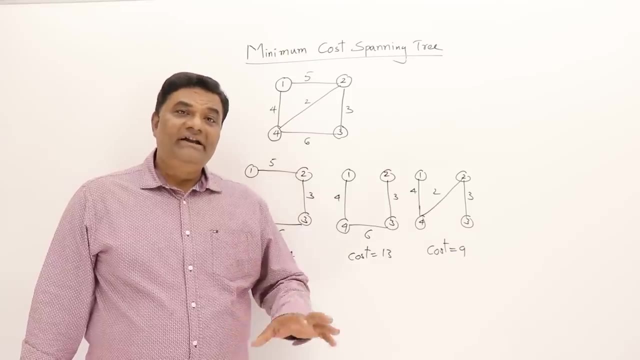 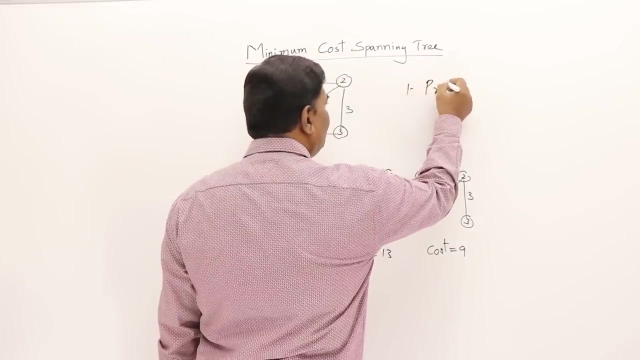 for finding the minimum cost spanning tree. if a weighted graph is given, you can find out the minimum cost spanning tree by following the method, without finding out all possible spanning trees. so what are those methods? one method is prim's algorithm and the second method is Kruskal's algorithm. 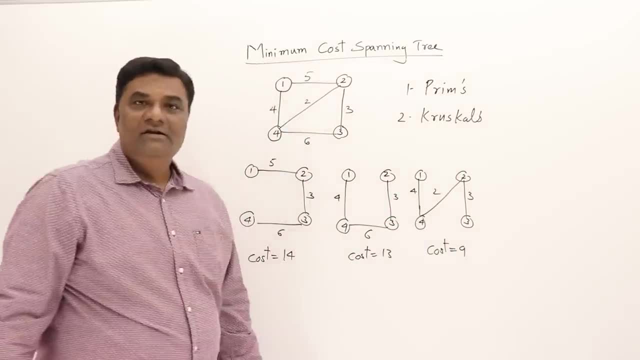 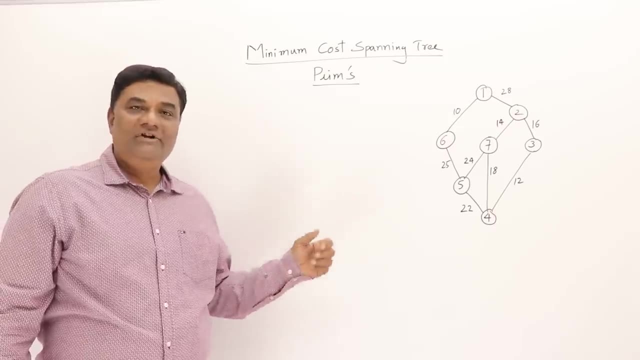 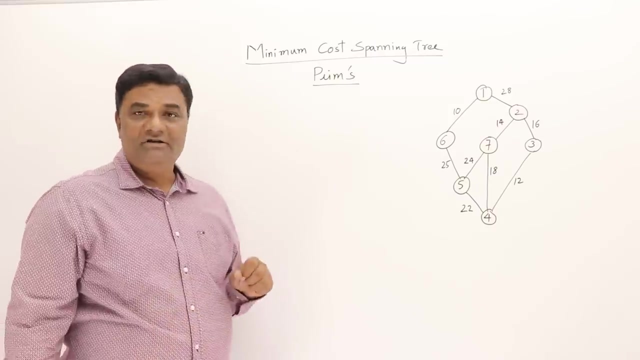 there are two algorithms for finding minimum cost spanning tree. I have a weighted graph here and I have to find a minimum cost spanning tree by following prim's algorithm. let's see how prim's algorithm works through an example. now, as per prim's algorithm- he says that from a graph. first, 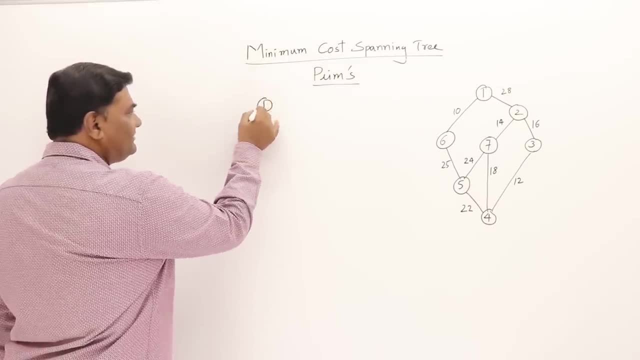 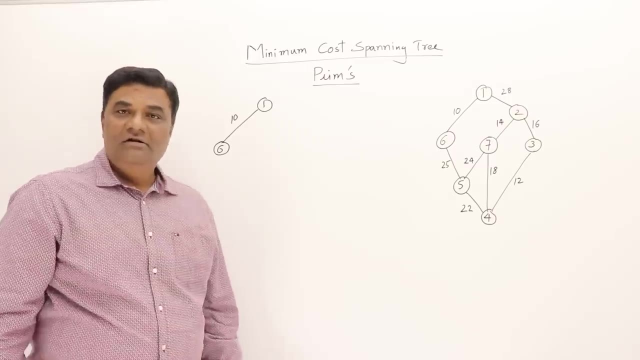 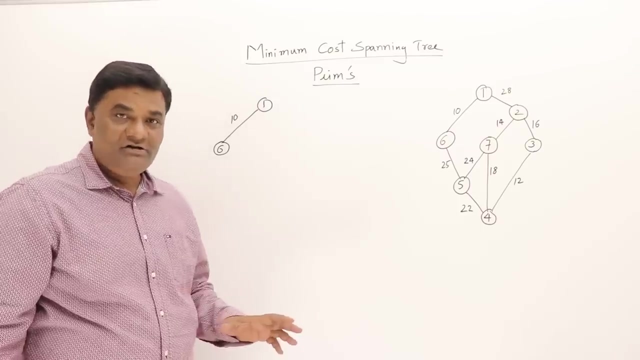 of all, you select a minimum cost edge, so the smallest edge in the entire graph is this one. so then, this is the initial one. now for the rest of the procedure. always select a minimum cost edge from the graph, but make sure that it should be connected to already selected vertices. 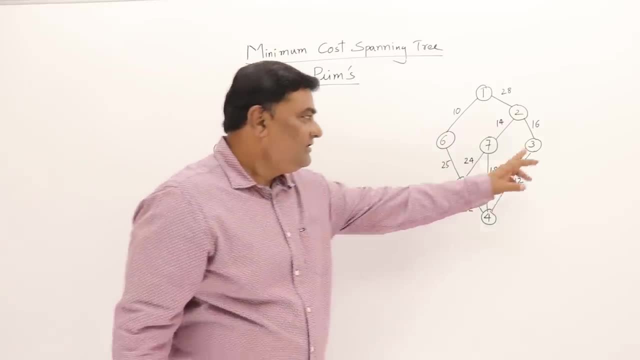 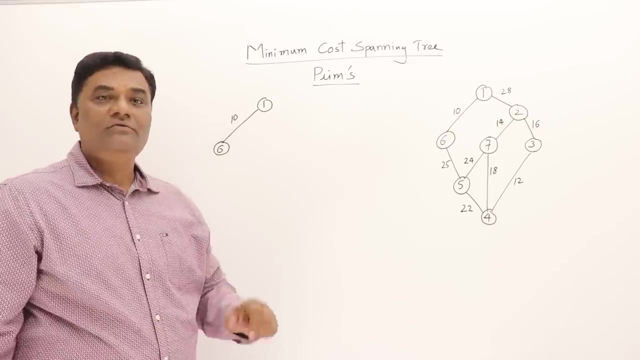 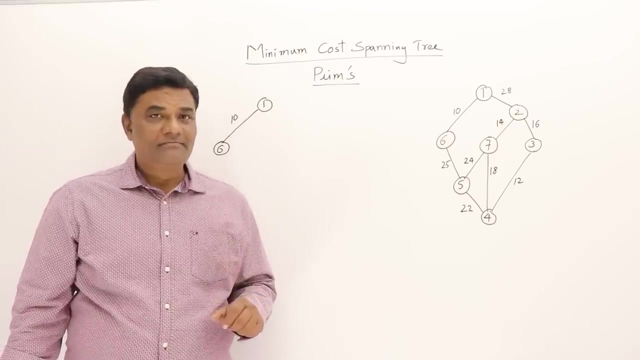 now the next minimum is which one? three to four, don't take that it will not be connected to one or six, so take only those which are connected to one or six means what he is trying to do is always maintain a tree. prim's thinks that if some farther away edge is selected, then 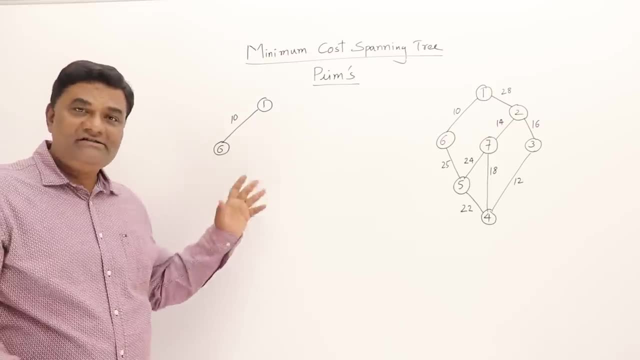 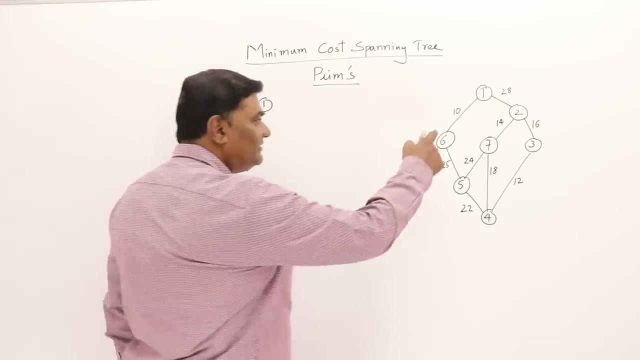 it may not be forming a tree. finally, so that is the reason he suggested that always select a minimum edge which should be connected. so let us see what is the next one. so for this connected one are this one and this one. so out of this, 25 and 28, 25 is minimum, so select. 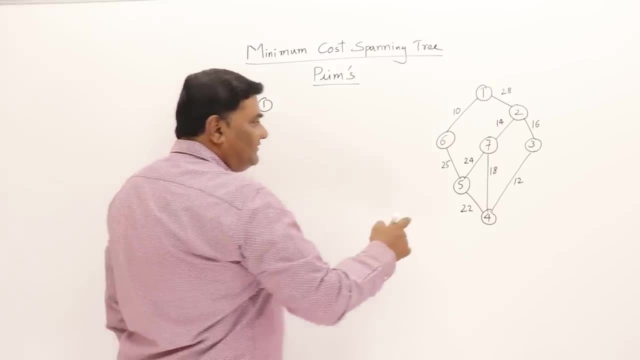 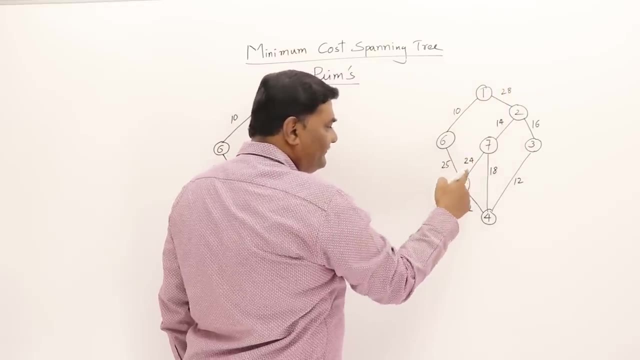 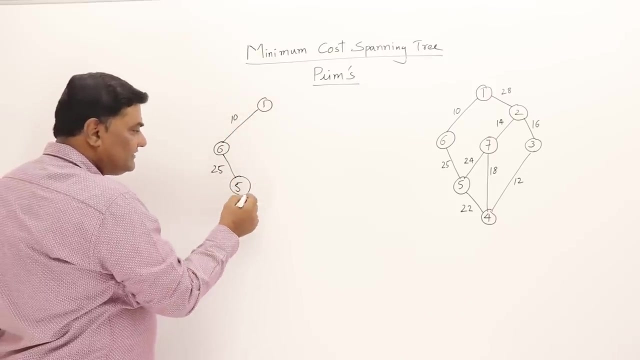 this 25.. then this 28 and 5 connected to 5 are 22 and 24. so out of this 28, 24 and 22, so from 1 and 6 and 5- i am checking so already- 6 is over, so 1 and 5, so out of those this is smallest one, so 4 is. 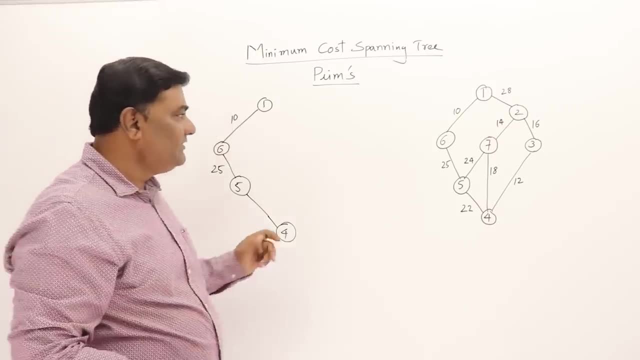 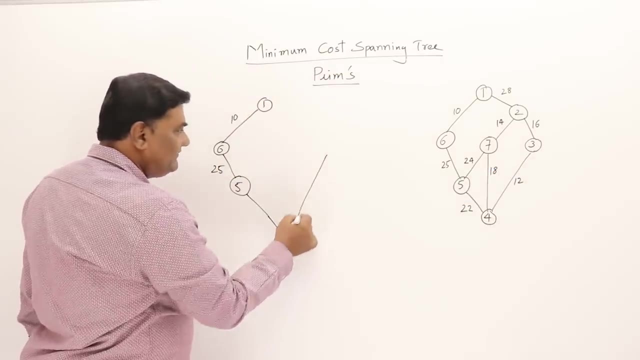 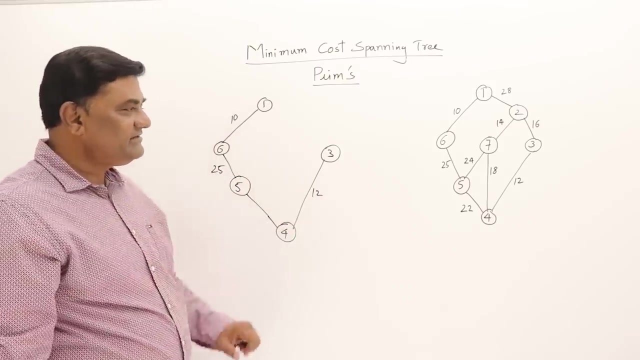 selected now from 1, 6 and 5, 4. who is smallest? the connected one, so this is 24 and 18 and 12, so 12 is a smaller. so we will take 12 then out of all these which connected as the smallest. so here i. 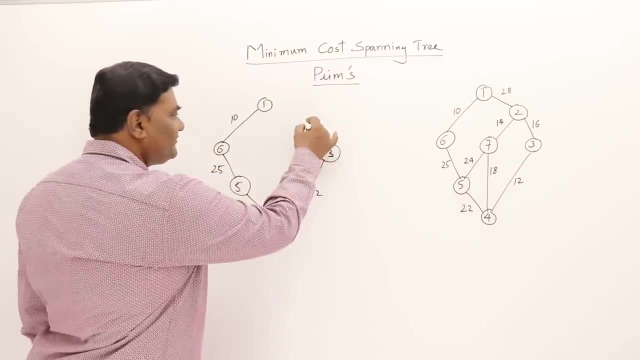 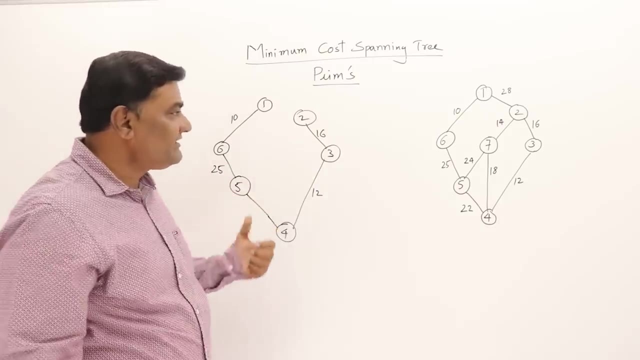 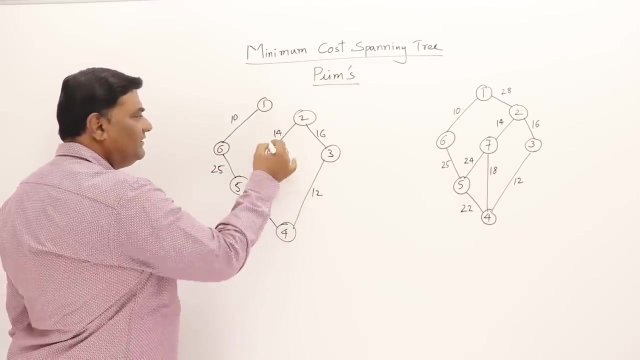 have 24, 18 and 16. so 16 is a smaller, so take that 16, then an out of all these. who is next connected? so from 2 to 7, there is an edge which is connected. so this is 7. that's it. 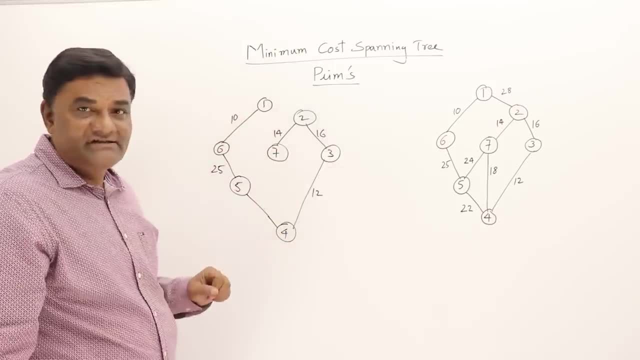 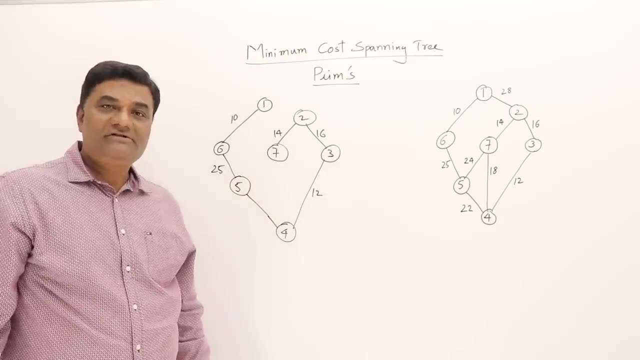 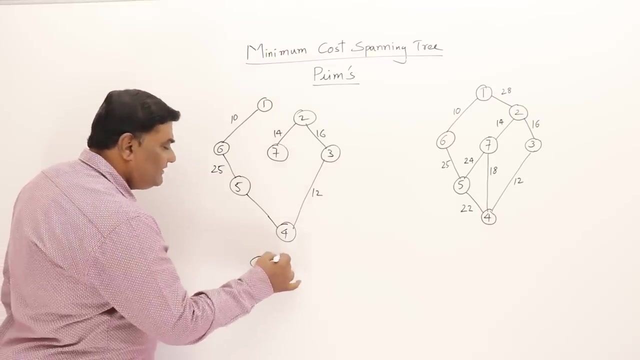 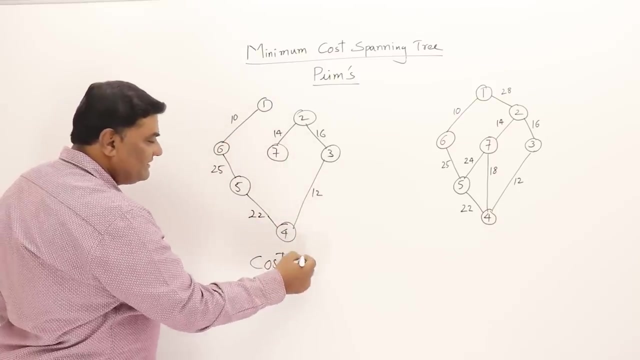 so there are seven vertices, so one, two, three, four, five, six, six edges are selected and this is how we got a minimum cost spanning tree. and and this is how we got a minimum cost spanning tree. what is the cost of a tree? the cost of a tree is if i add all these. if i add all these, it is 99. 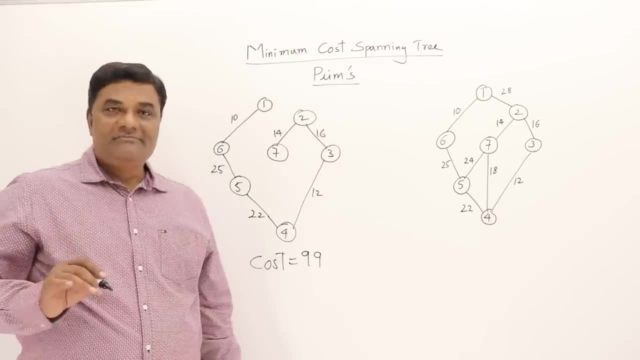 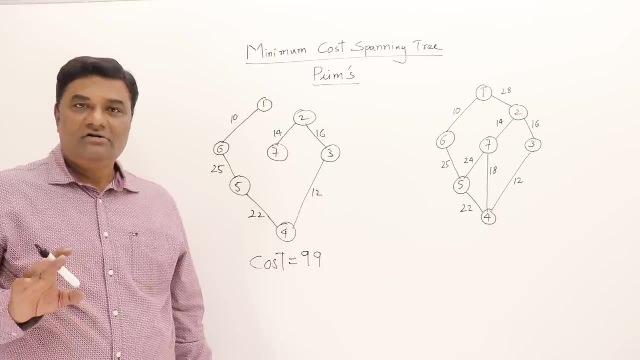 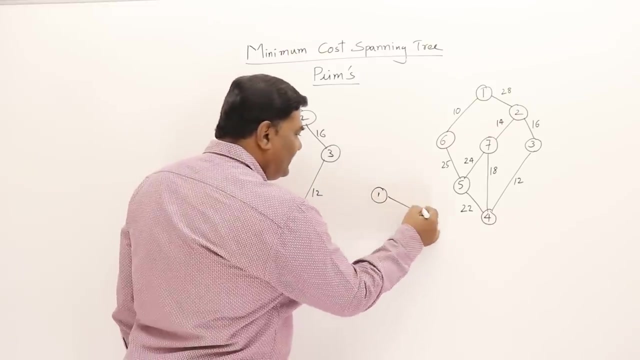 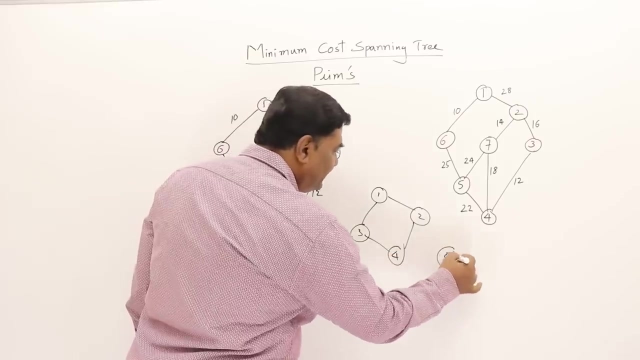 so the approach of premises: initially select the smallest one and then we will take the minimum cost spanning tree and then we will take the smallest one, then always select the connected smallest one. all right, so this is the method of prime shell for them. next, if i have a graph, one, two, three, four, five, six, seven. if i have a graph, 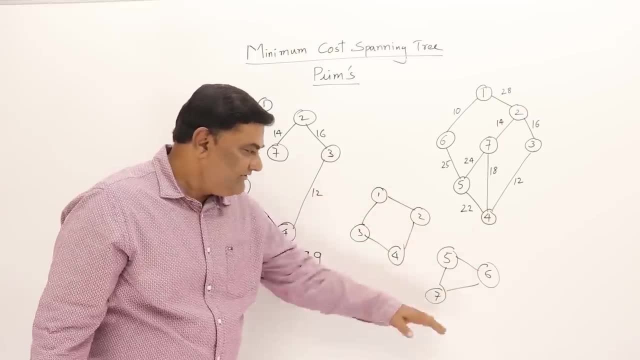 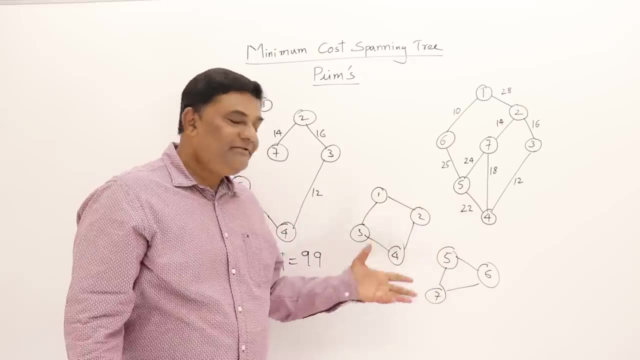 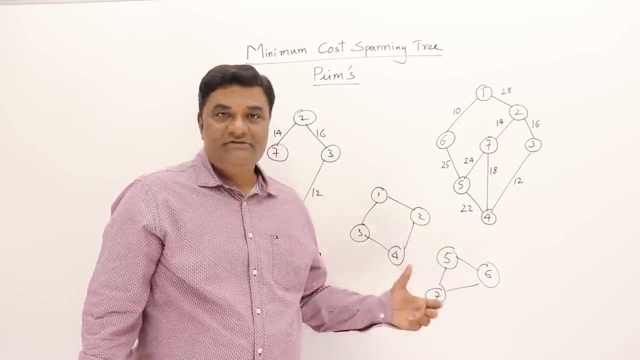 like this, which is not connected. there are total seven vertices but there are two pieces in a graph. can prim find out the minimum cost spanning tree for this one? no, no algorithm can find out because we cannot find a tree for this one spanning tree for this one in a spanning tree. it must be. 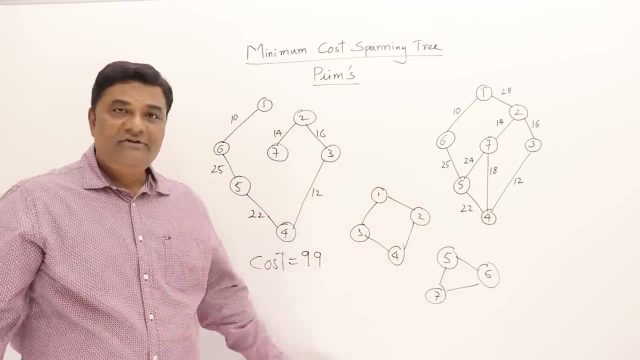 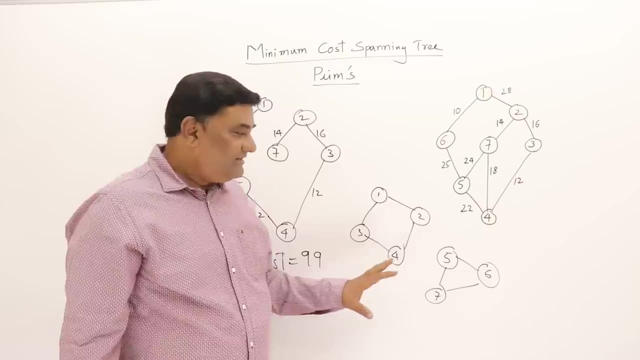 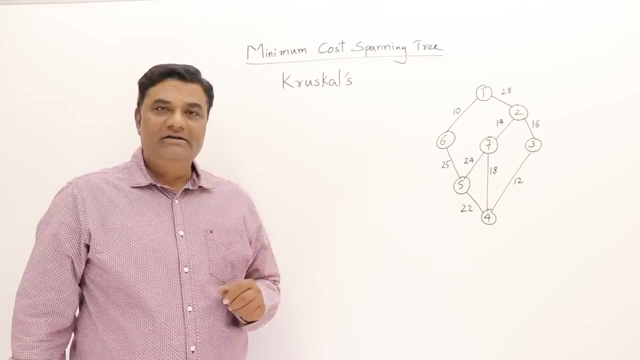 connected. so for non-connected graph we cannot find spanning trees at all. but if i start prims on this one, starting from vertex one, if it is starting, then it may find the spanning tree for only one component, not the other component. next method for finding minimum cost spanning tree is kruskal's method. this also follows a greedy. 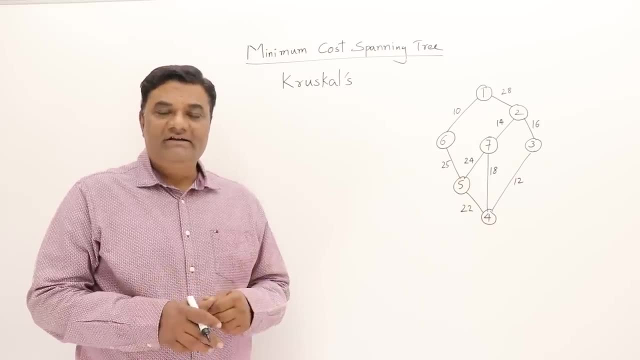 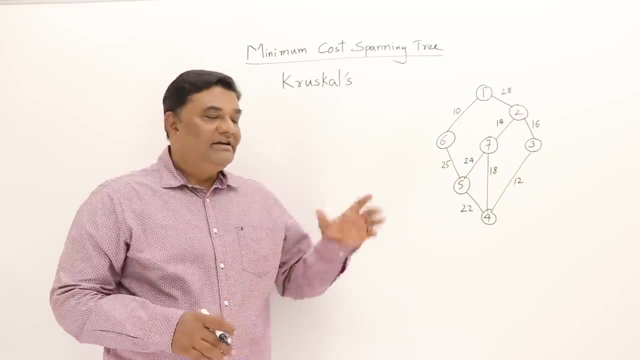 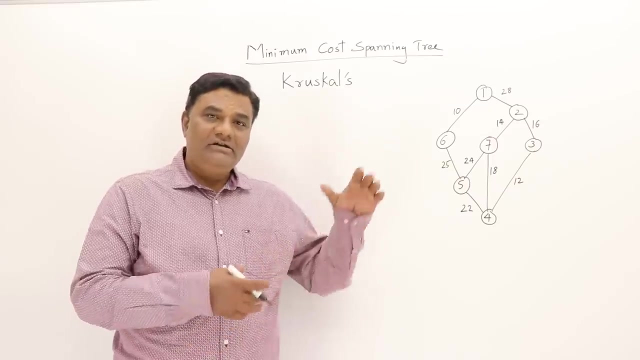 approach. instead of trying out all possible spanning trees, it shows a procedure by following which we can get a minimum cost spanning tree. it says that always select a minimum cost edge. always select a minimum cost edge. let us follow this one. let's select smallest edge. one, two. 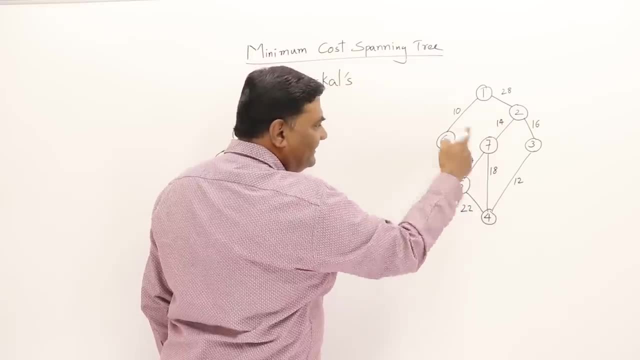 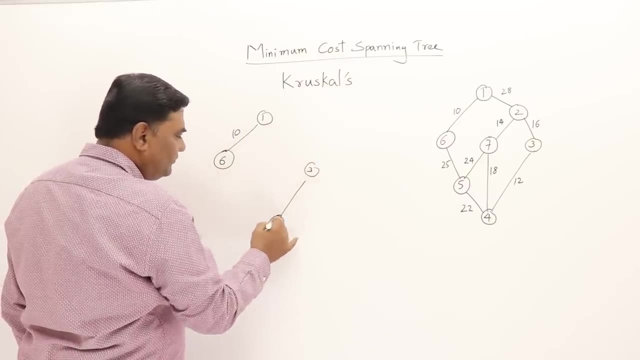 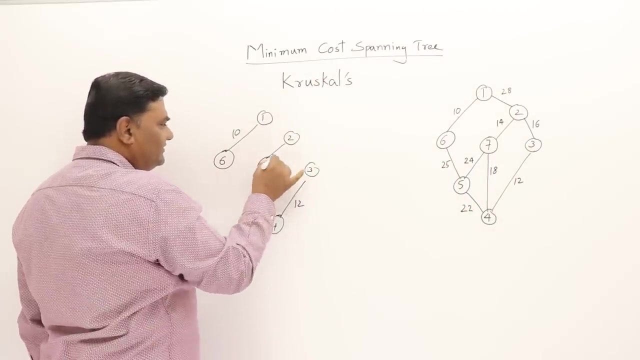 six, that is 10. this one is the smallest and the next smallest test is 3 to 4. so the second edge and selecting is 3 to 4 and its cost is 12.. next minimum is 2 to 7, select 2 to 7 and this is 14. 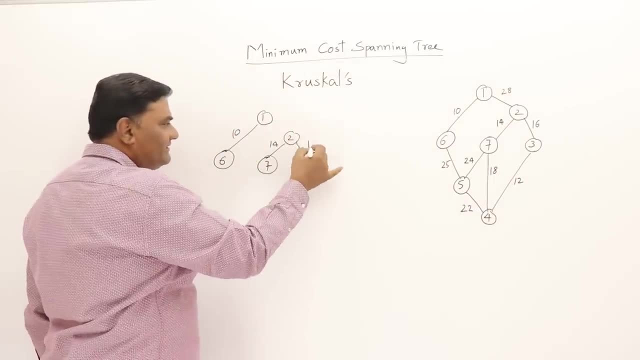 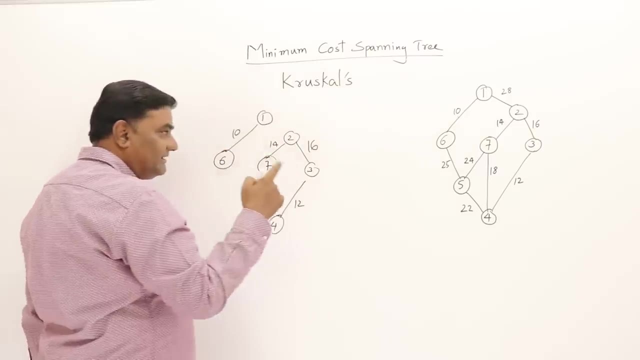 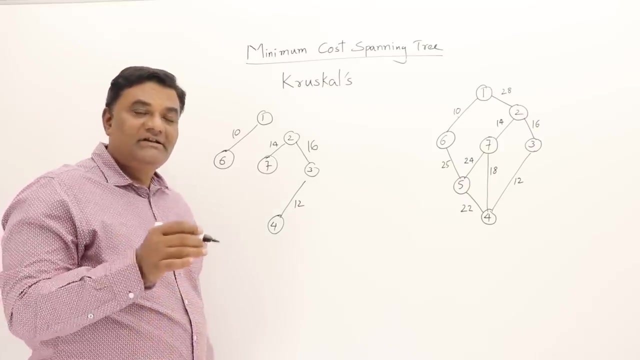 and the next minimum is 2 to 3, that is 16.. and after this the next minimum edge is 7 to 4, but but that is 18. if I select that, it will form a cycle. yes, Kruskal method says that, always select. 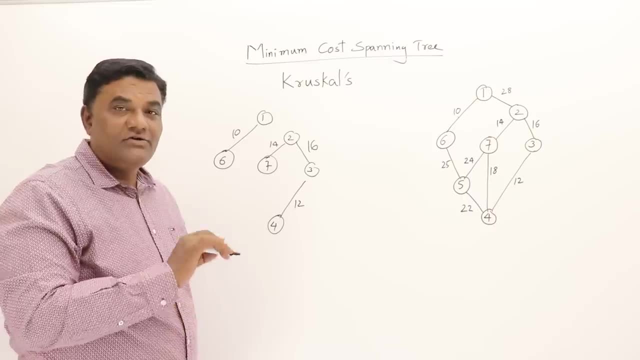 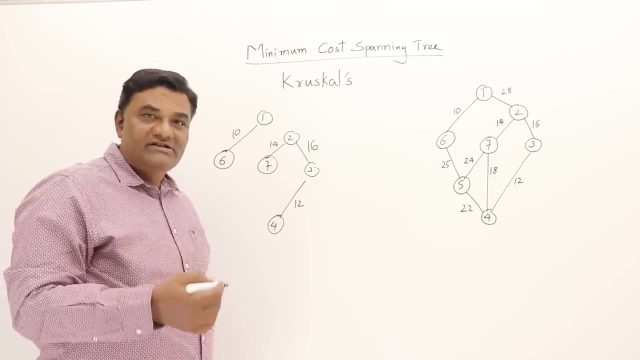 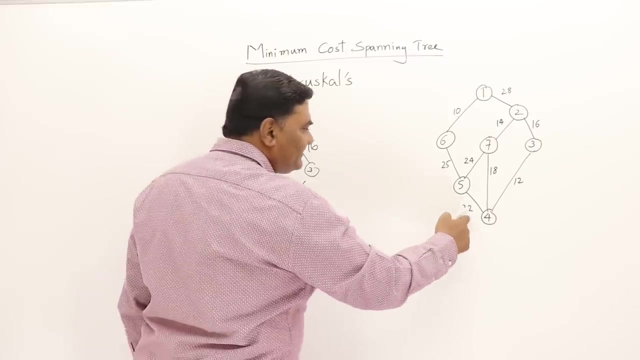 a minimum cos h, but if it is forming a cycle don't include it in the solution. discard that h don't include an h. so it means always select such that it is not forming a cycle. so if I include 4 to 7 it will form a cycle. so next one you check. so the next one is 22, so this is from 5 to 4, or 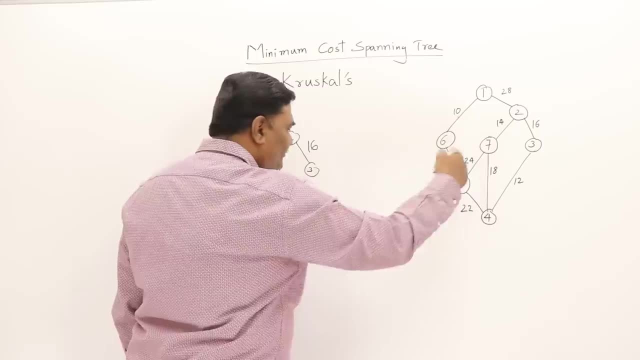 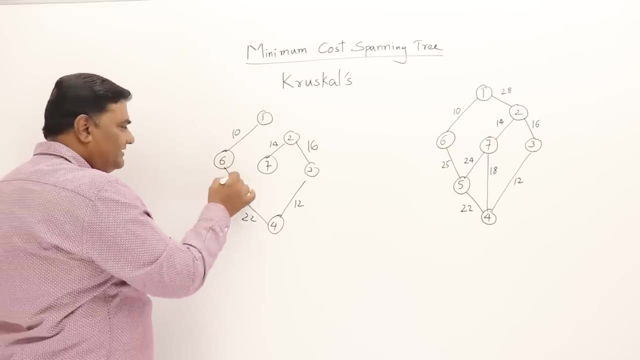 4 to 5, so this is 22. next minimum is 24, so that is 7 and 5. if I include this also, it will form a cycle. don't include that one. then the next minimum one is 25, that is, from 5 to 6, so this: 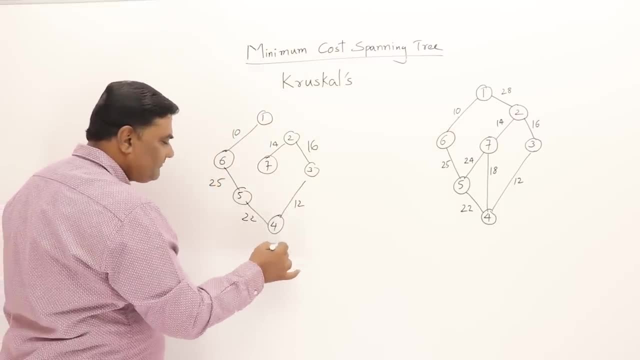 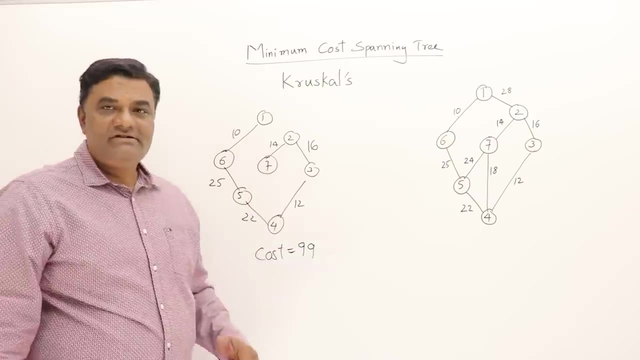 is 25 and the cost of this one is: if you add all these weights it's 99. so here also I got the same result, just how I got in Prim's algorithm. so the Prim's algorithm and Kruskal algorithm have the same result. just how I got in Prim's algorithm. so the Prim's algorithm and Kruskal. 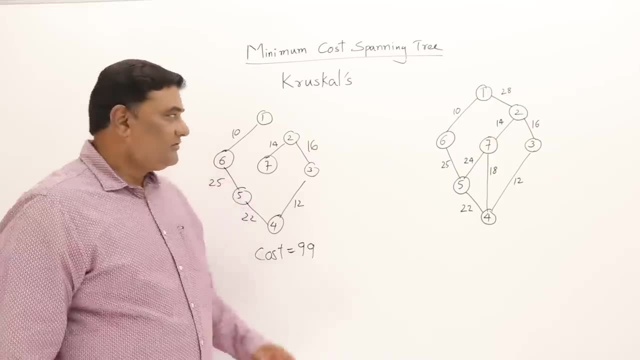 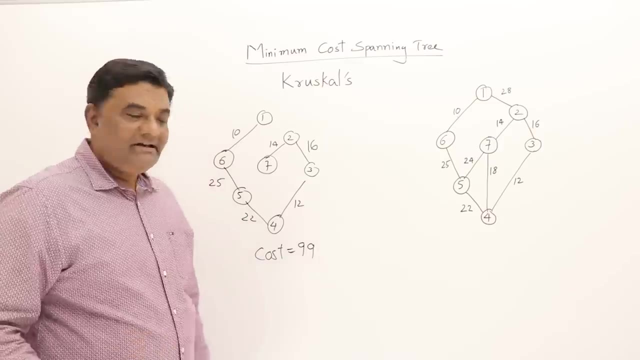 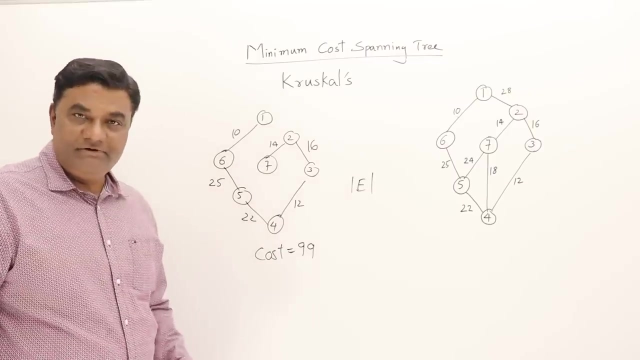 has given the same result on this particular graph. now, time taken by Kruskal's algorithm. how much time it takes? see it has to always select a minimum cos h from the set of edges. so let us say there are e number of edges, so out of these edges it will find out the minimum one. 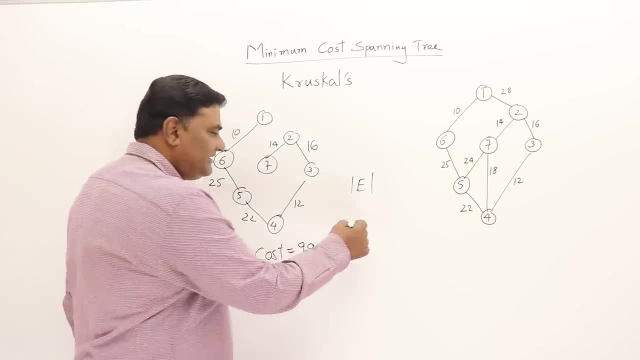 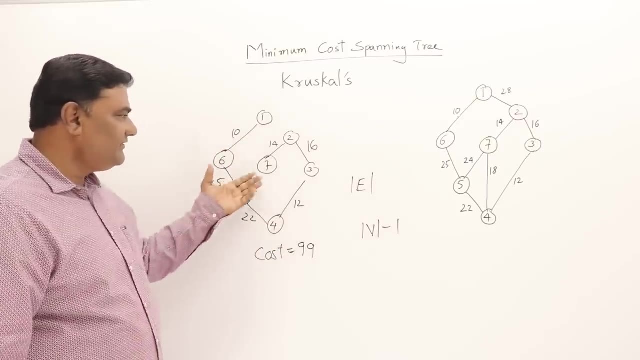 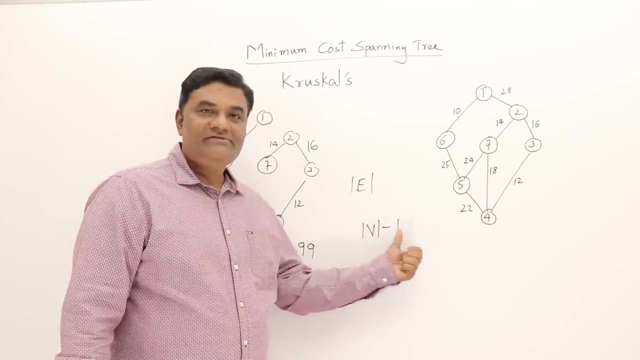 and how many such edges it will be selecting. it will be selecting v minus 1. yeah, this number of vertices minus 1. so, like we know, in a spanning tree if there are seven vertices we need six edges for forming a spanning tree. so that's 7 minus 1. so as many vertices we have minus one. 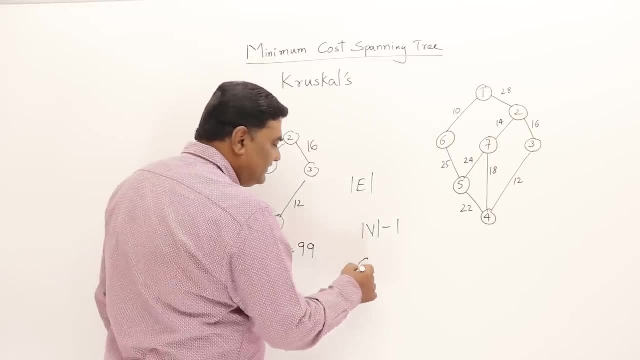 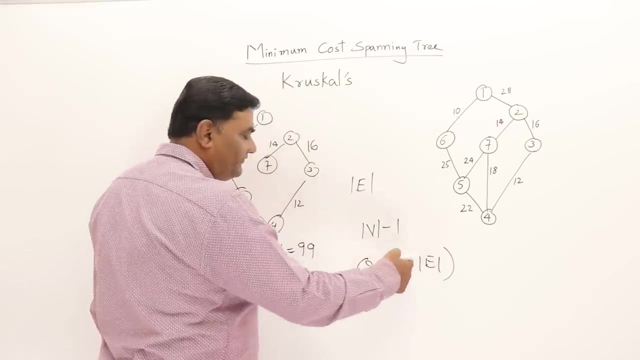 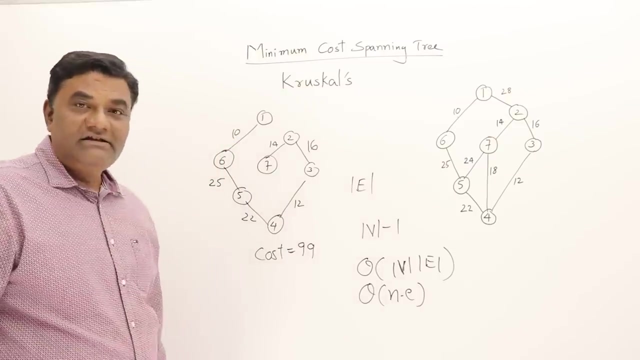 number of edges we have to select. so the total time will be theta of v into e. there e v is number of vertices and e is number of edges. so it is n into e. n is the number of vertices and e is the number of edges which can also be written as n squared, if we say both are equal to n squared. so 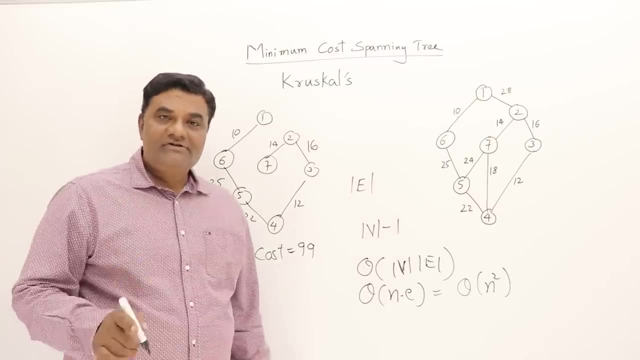 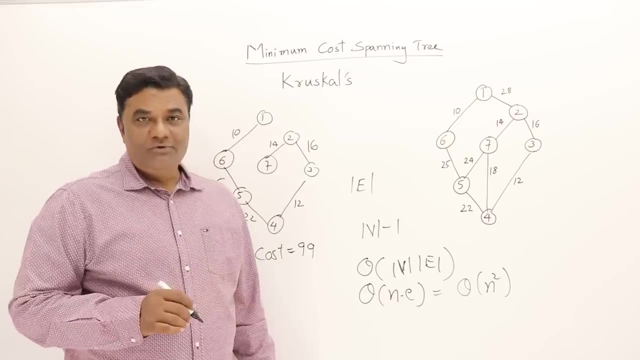 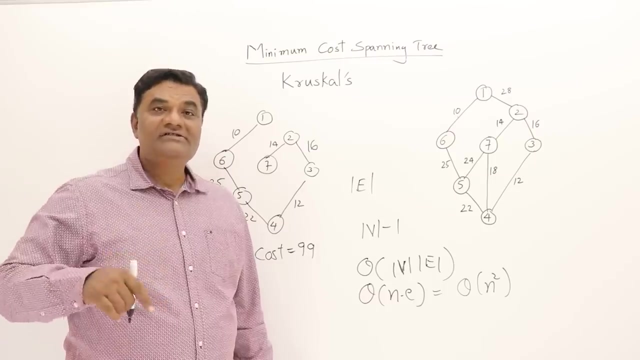 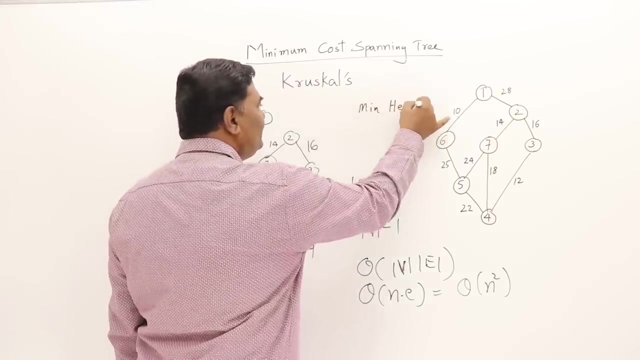 it is n? squared, so the time taken by Kruskal's algorithm is n? squared. but Kruskal algorithm can be improved. when we have to always select a minimum cos h, then there is one data structure which will always give you minimum value. that is min heap. if min heap is used, then min heap will. 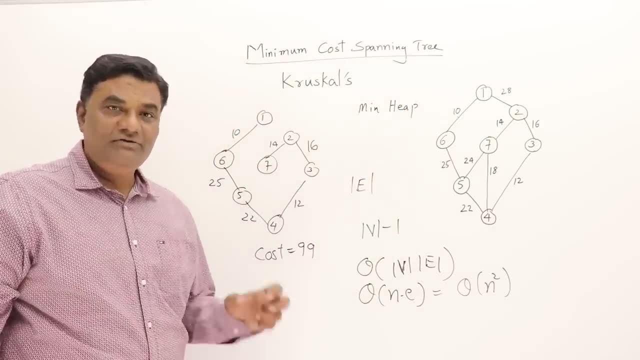 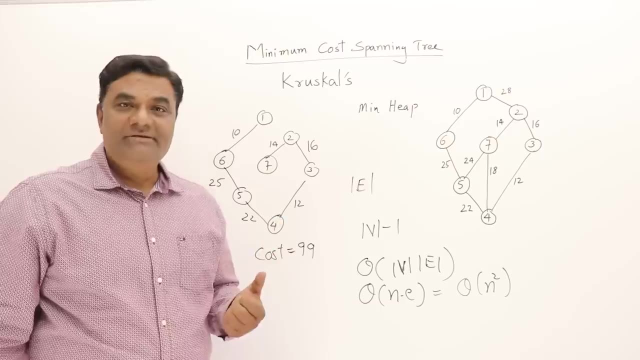 always give you a minimum value. whenever you delete a value, you get a minimum value. so if all these edges are kept in a min heap, whenever you delete you will be getting a next minimum edge, so you don't have to search so from min heap. whenever you delete, the time taken is 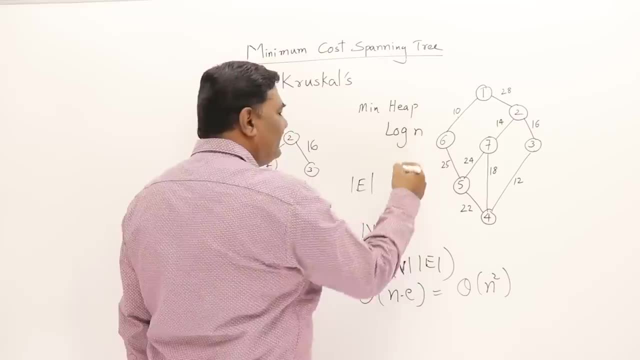 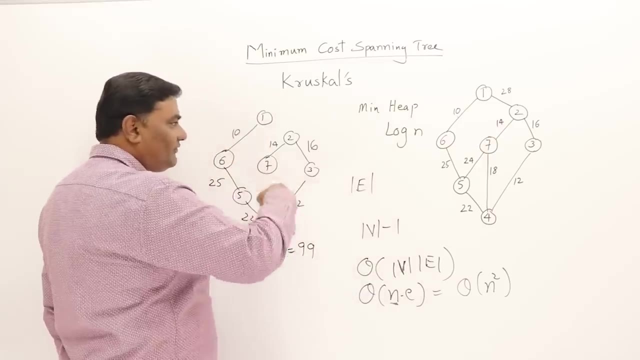 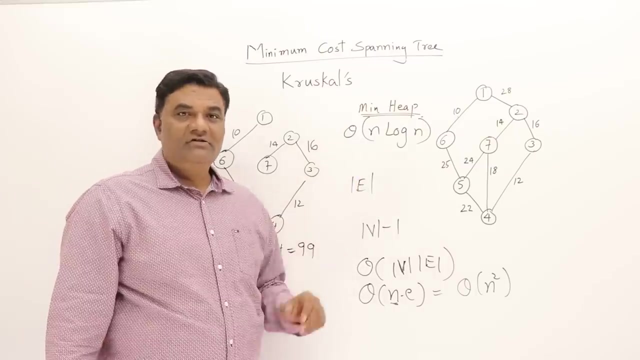 log n. so how much time it will take for finding a minimum cos h log n time. so how many times you have to do that. that is n time. number of vertices minus one time, so n. so by using min heap, the time time complexity of Kruskal's algorithm will be n squared. so this is the time taken by Kruskal's. 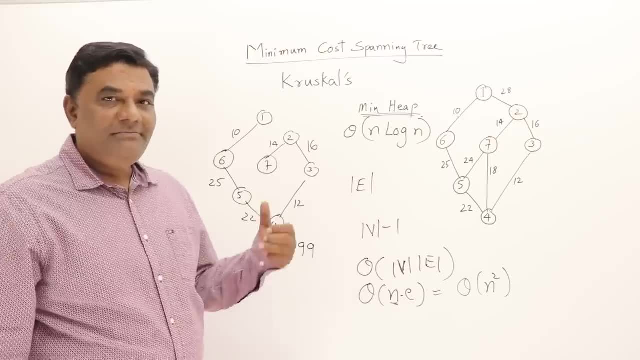 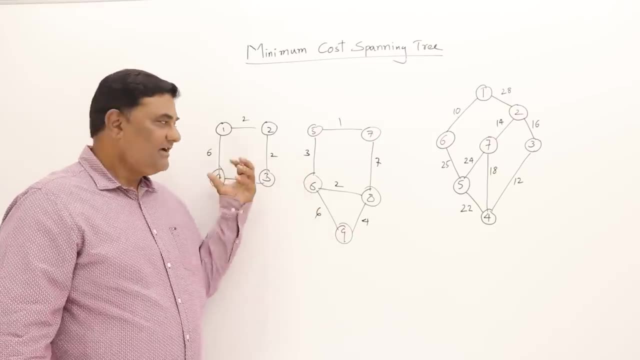 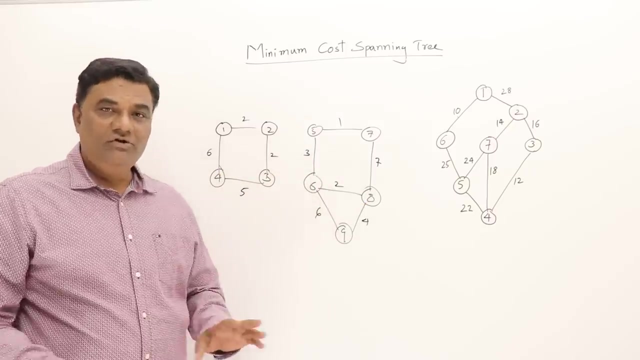 algorithm log n. so that's how Kruskal's algorithm can be made faster. now, if there is a graph given that is not connected graph, it is having two components: four vertices on this side, five vertices on that side. can we find a spanning tree on a non-connected graph? no, spanning tree is not. 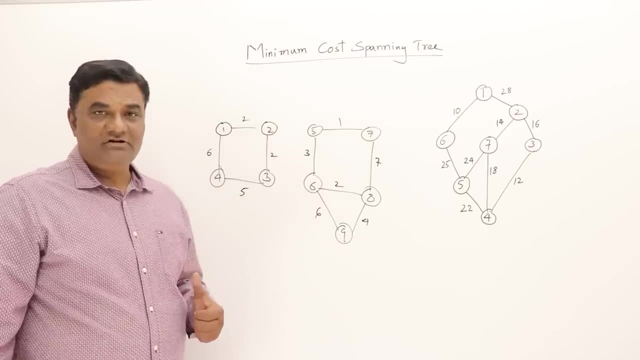 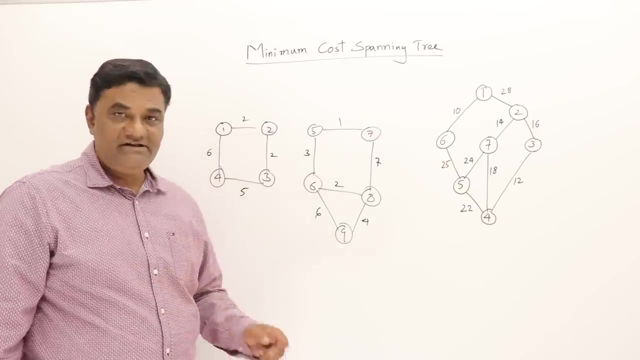 possible. but what happens if I run a Kruskal's algorithm? so Kruskal's algorithm will try to find out total number of edges that is nine minus one. so it will try to select eight edges and it will not be forming a spanning tree for entire graph, but it may be finding the spanning. 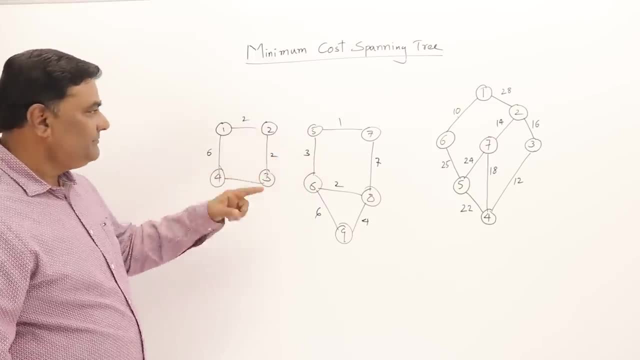 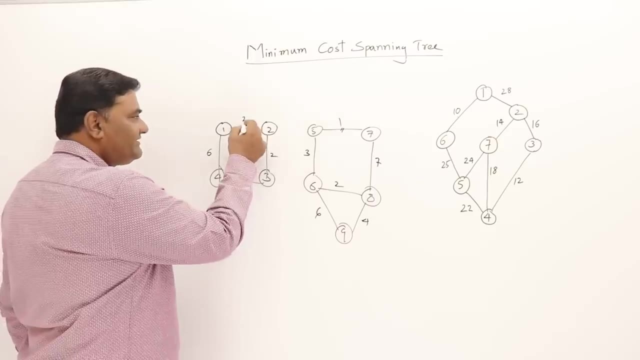 tree for each component. let us say, if the first minimum, the one it will select, is this one, then the next minimum it is having more than one edges. let us say it selects next minimum and the next minimum it will select this. next minimum, it selects this and this is the next minimum. so in this way, 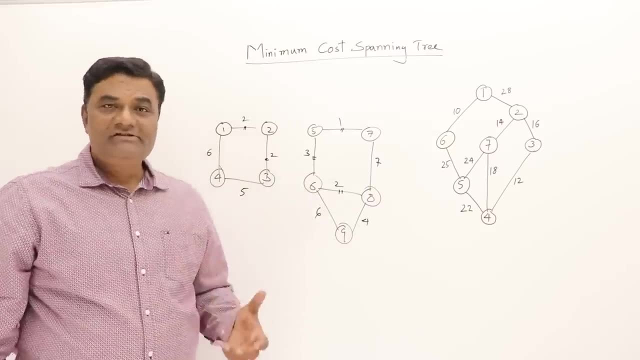 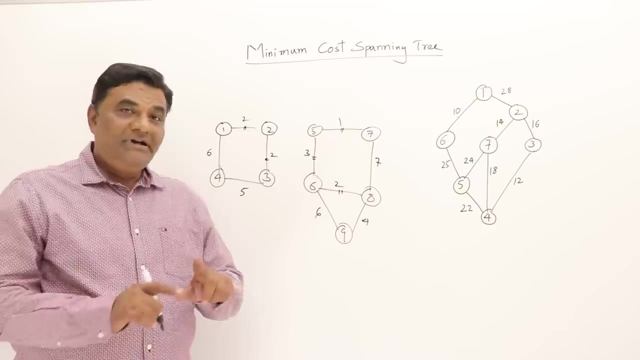 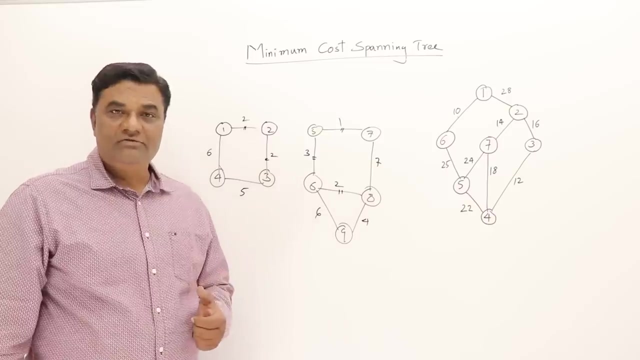 it is selecting the minimum edges from both the components or it will be selecting from all the components, so it may be finding spanning trees for all the components but not for the entire graph. so Kruskal's algorithm may work for non-connected graphs also, but it may give spanning. 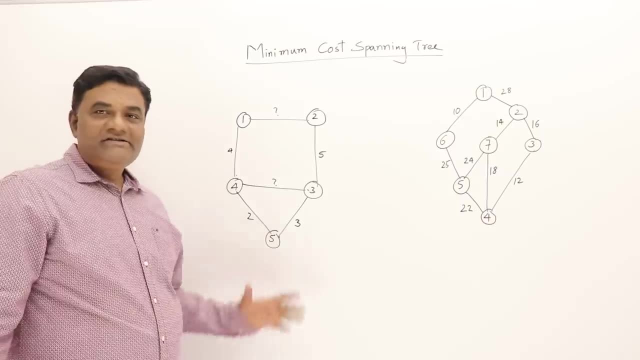 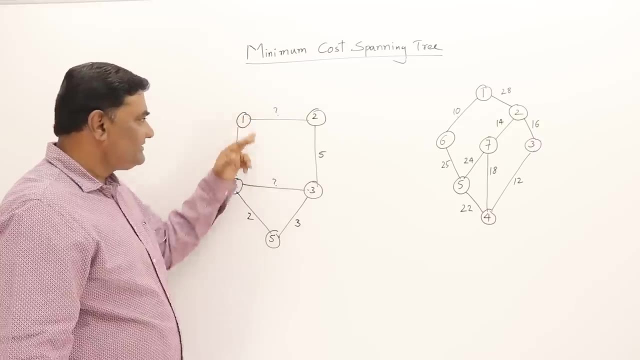 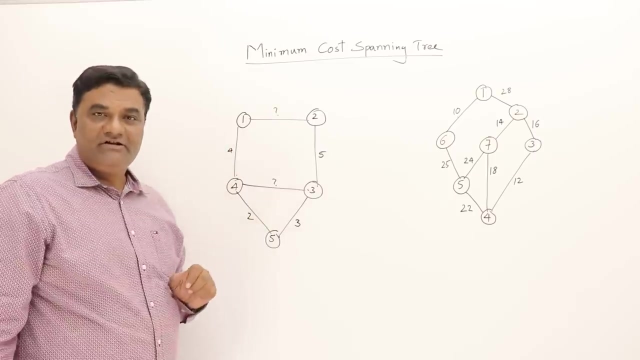 tree for those components. let us take a problem here. a graph is given and the weights of the edges are also given, but here two edges are not having their weights. if I take only these edges, which are eight, they are forming a spanning tree of a graph. just hide these two edges, it becomes a spanning. 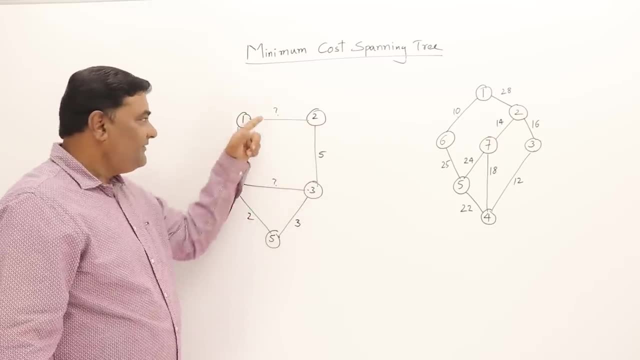 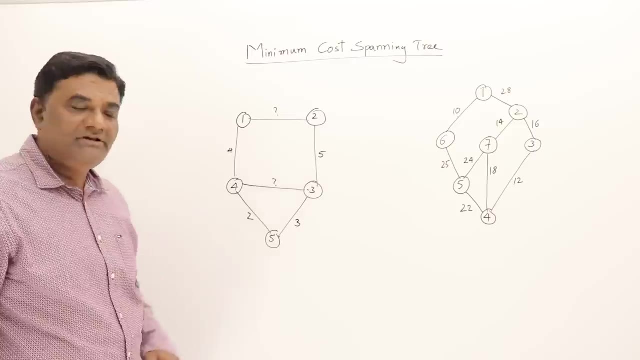 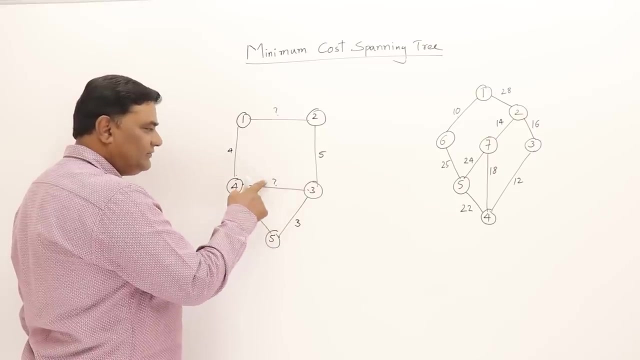 tree. now the question is: what could be the minimum values of these two edges? what could be the minimum possible value? maximum, it can be anything, but at least what could be the value. see, as this is included in a spanning tree, this is included in a spanning tree. this is not included because it. 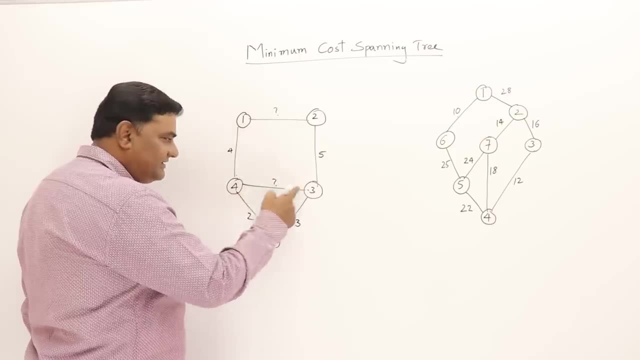 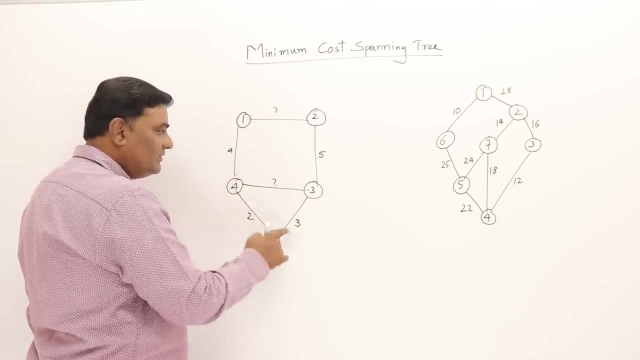 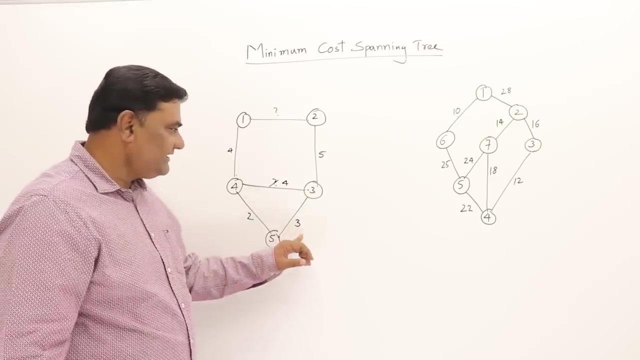 is forming a cycle. so it is forming a cycle. if it is included, this will form a cycle, so it may be considered. after selecting these two, after selecting these two. so the weight of this could be four right: first this is selected, then this is selected, then this is not selected. means: 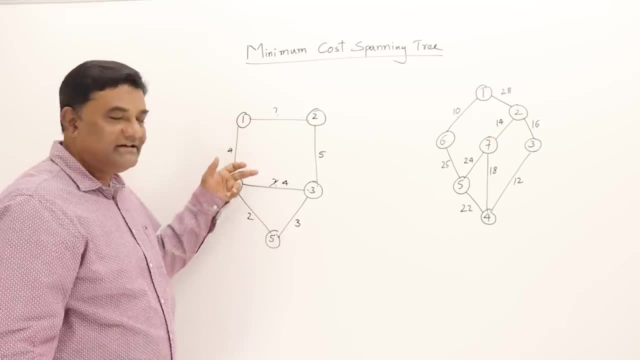 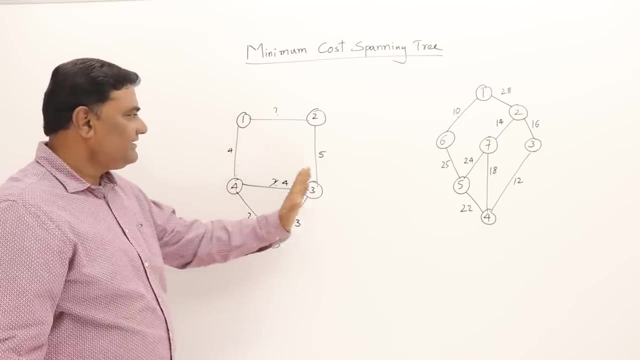 definitely it is four. if it is less than four, then that would have been selected first, right, so it came later. so it is forming a cycle. so it is not taken, then this four is taken, then this four is taken, this five is taken. so then what could be the minimum weight of this one? so it 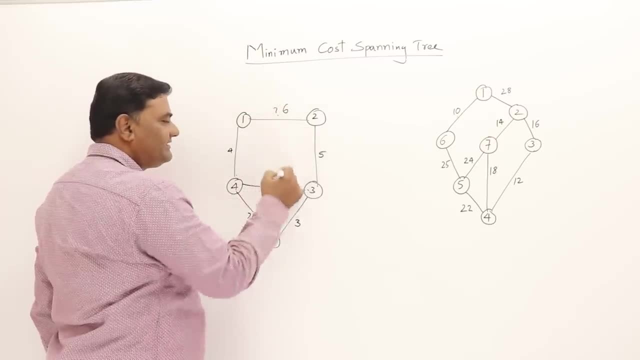 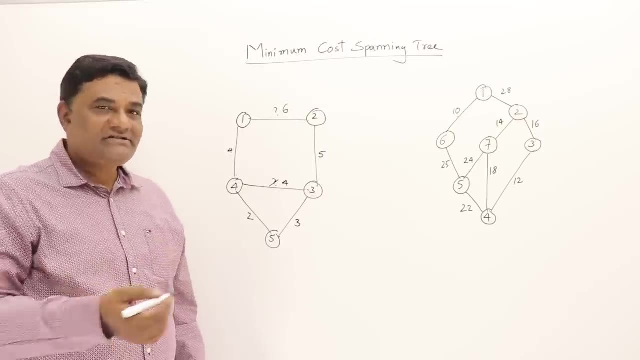 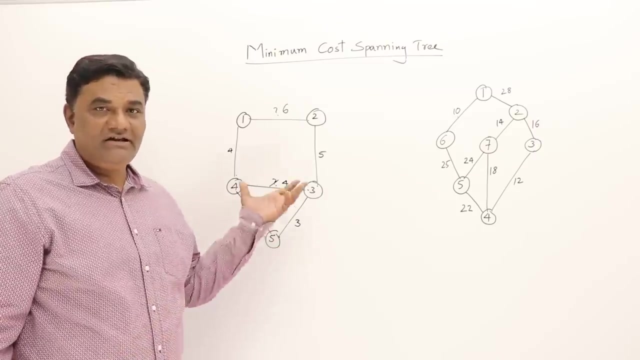 at last it is left over- means minimum weight of this one could be six, so this is four and that is six. so if any missing edges are there you can find out. this type of problems we find in examinations. so some missing edges you can find out. so if you know spanning tree you can answer this type of 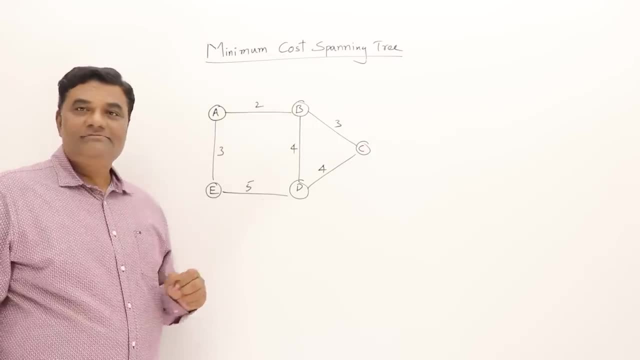 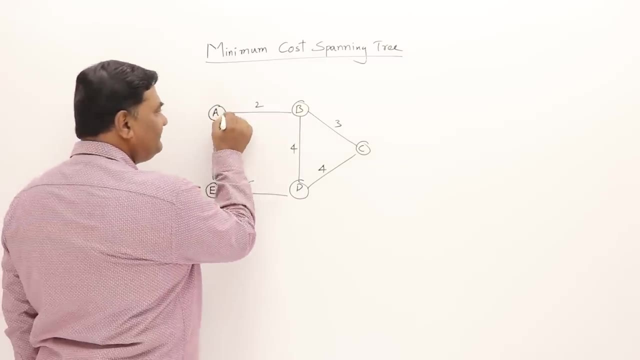 question. let us take this example and let us find out: spanning tree for this one minimum cause spanning tree. so if I follow Kruskal's method, so first I will select the minimum cause edge, this edge I have selected, then the next minimum is this three and that three, so I can. 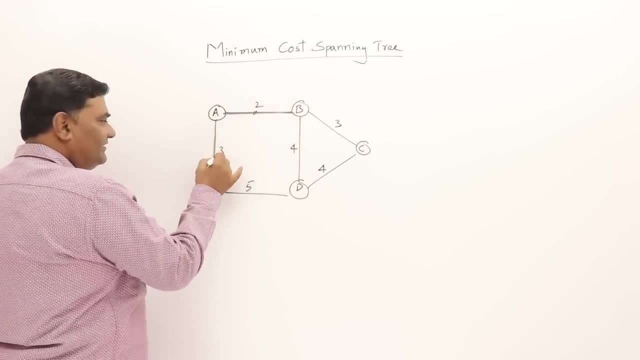 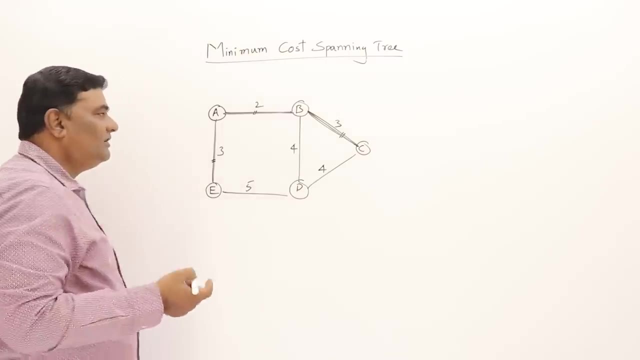 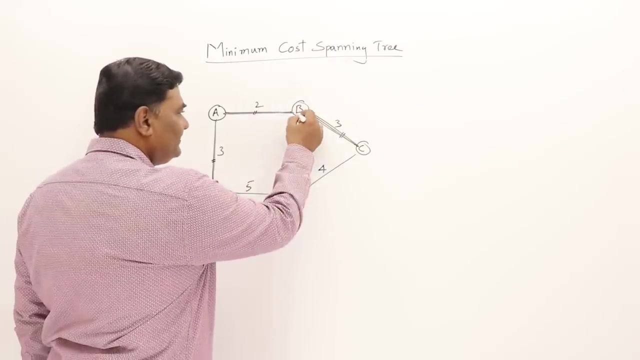 select any one, so I will select this one first. this is selected, next I will select this one. so is it forming a cycle? inclusion of this one? no, so I will select that one. then which other edges? four and four? these two are there, so I can select any one, so I will select this one. 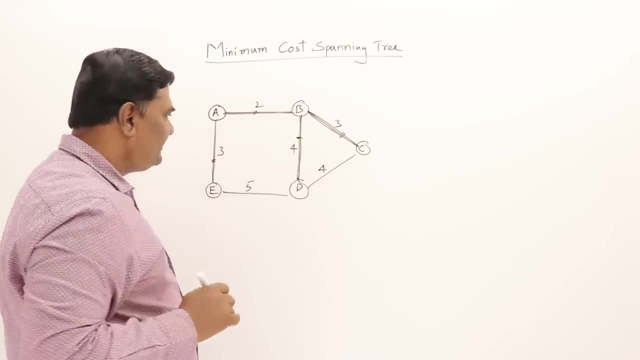 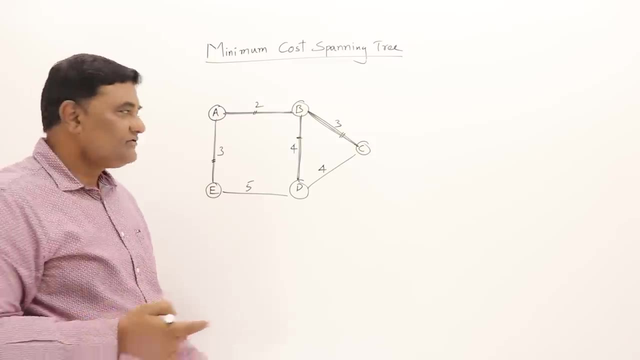 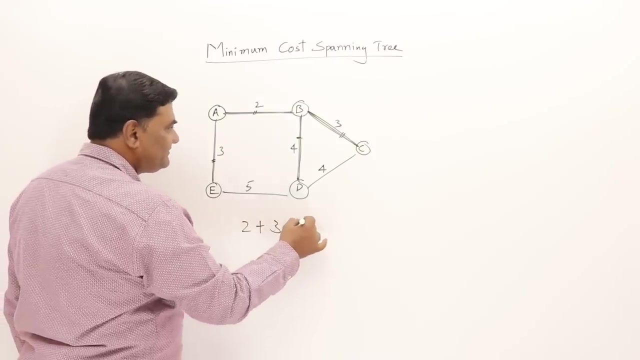 whether this will form any cycle. no, so total how many edges I have selected. one, two, three, four and total how many vertices are there? five vertices are there, so four edges are selected. that's how I got a spanning tree. so what's the cost of the spanning tree? two plus three plus. 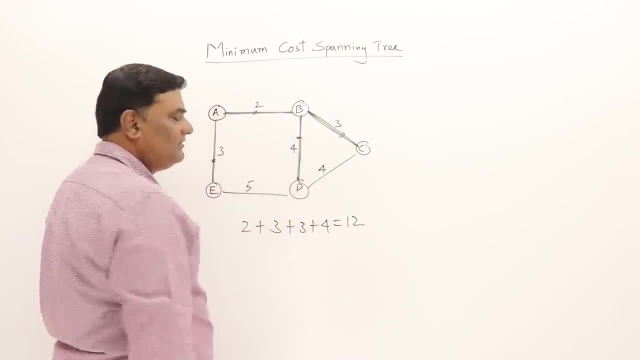 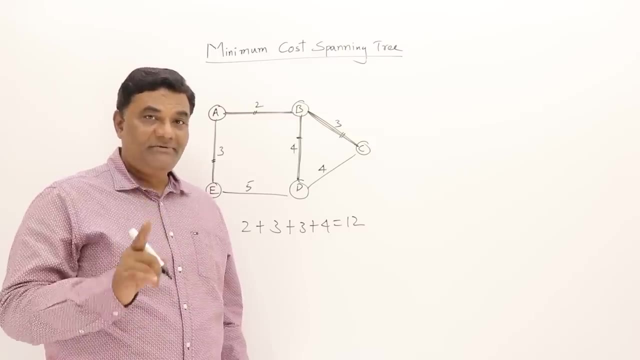 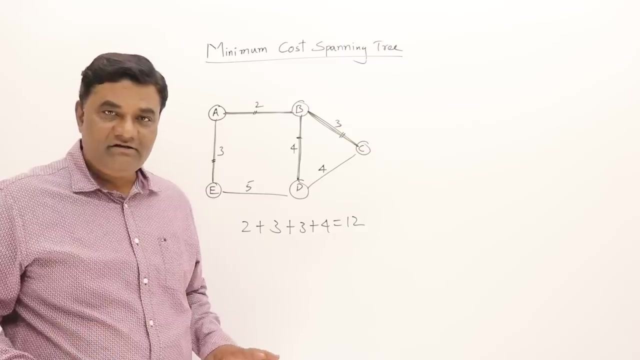 three plus four and this is two. nth spanning tree is a minimization result, so definitely there will be only one result. so for a problem there can be only one optimal solution. so we should have exactly one spanning tree. only there cannot be more than one spanning tree, right, but in this? 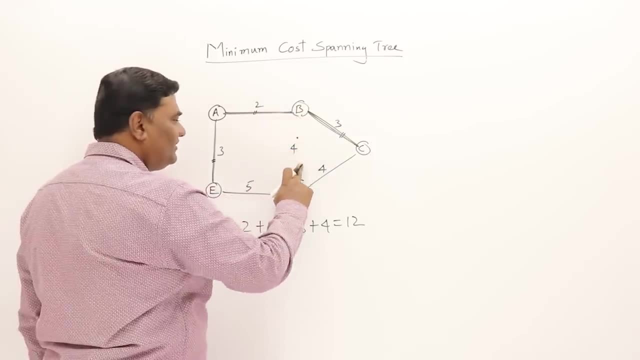 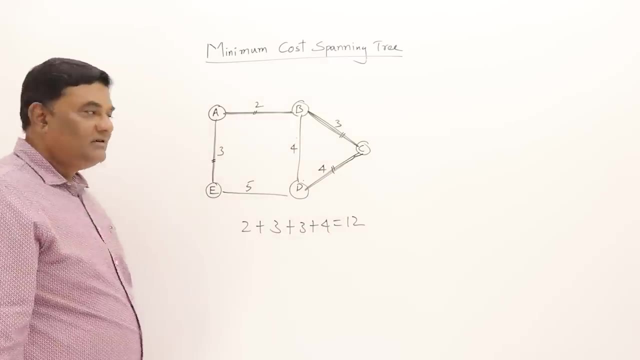 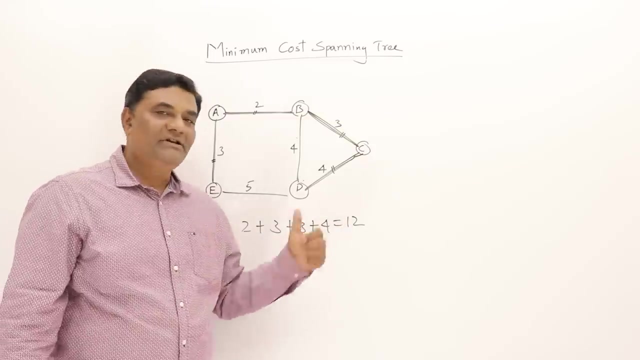 example, you can see, instead of taking this four, this edge, I can take this four also. now also it's forming a spanning tree. yes, so I can select one more, but what is the cost? cost is 12, so cost is only one. the optimal cost is 12 only. you will get definitely only one. 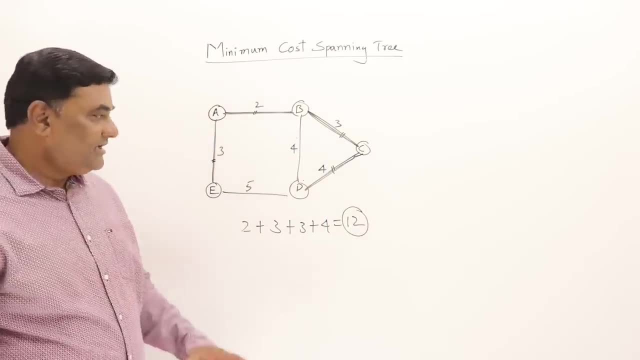 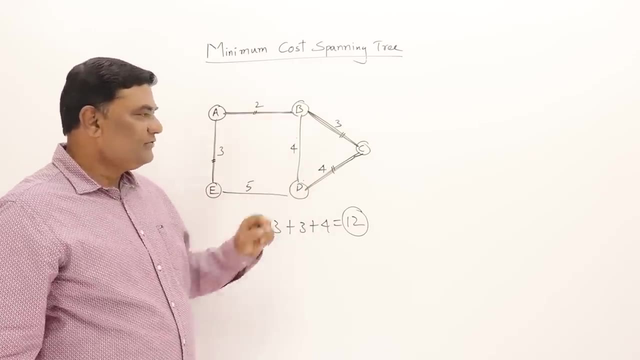 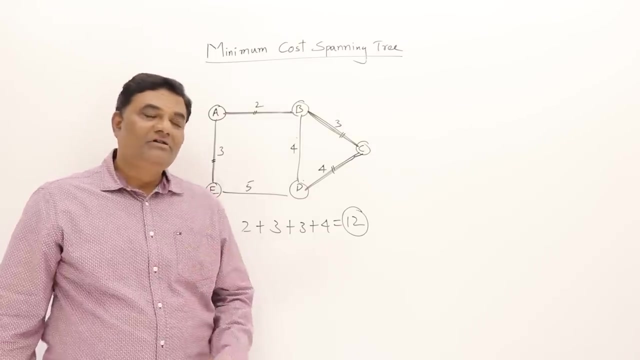 answer in the minimization or maximization problem. but for that answer the set of input is changing. so either you can include this four or this four. so total: how many spanning trees are trees are possible? two spanning trees are possible, but what is the minimum cost? that is 12..